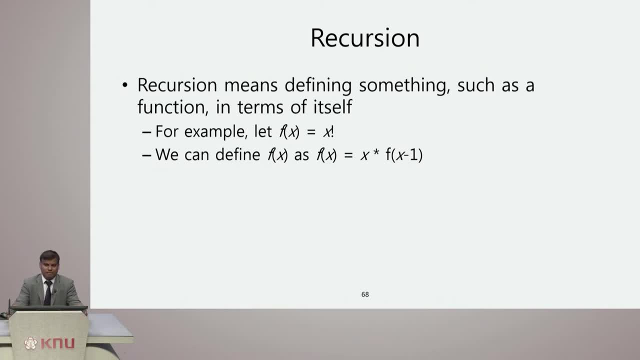 For instance, if you really want to do some repeated task, then you can go for a recursive function, because it just does the same thing again and again. Whenever you want to do that part, just call this function. We saw that is similar to the sequence as well. 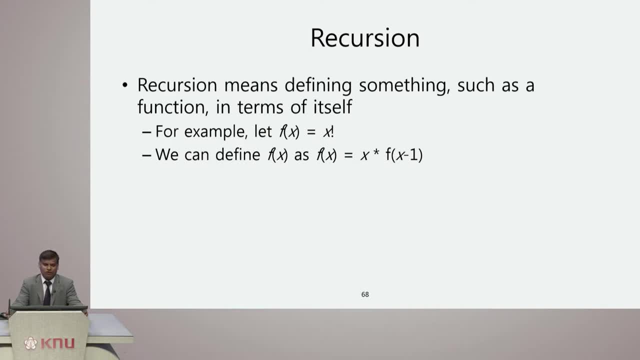 If you recall the sequence, we might have a for loop and then it repeats until that maximum limit. For example, if you have a summation and summation you have summation n equal to 0 to say x. 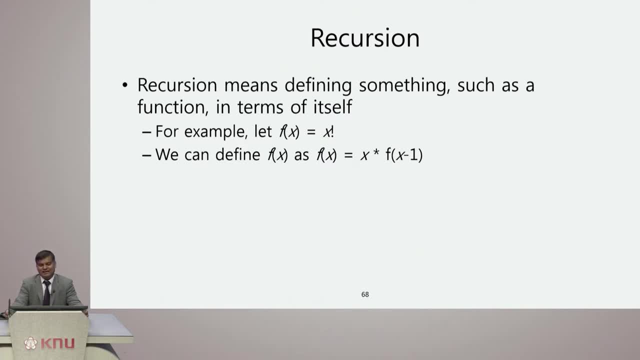 or x equal to 0 to n. In either case, you are going from 0 to a limit, And you always limit this by means of this, for example, using a for loop, Rather in case of a recursion, as you have written a function. 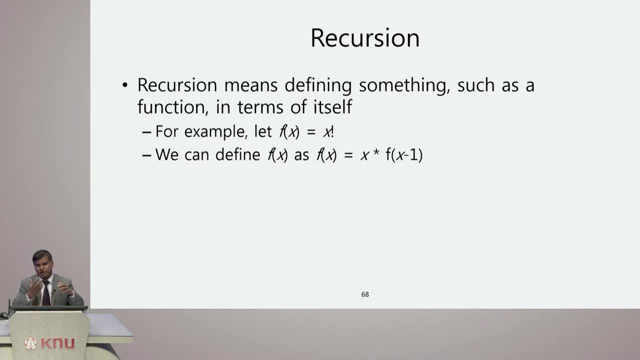 and this function. you can call this function again and again to itself until a condition is met, for example- And of course we'll see an example later on- And we should be very cautious of using this recursion because at times your system might get into a deadlock condition: deadlock. 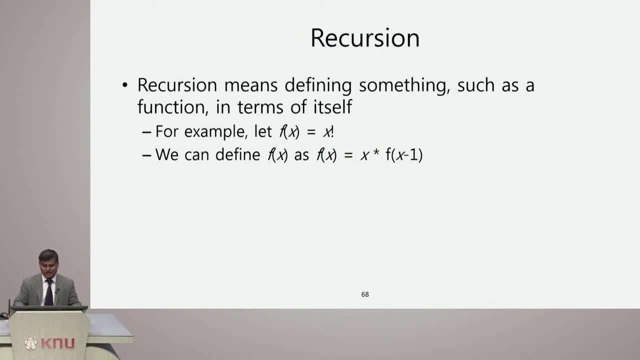 We'll see about that later on. Let's talk more about this recursion. Let's see a few examples of recursion here. We are asked to find f of 1, f of 2, f of 3, and f of 4. 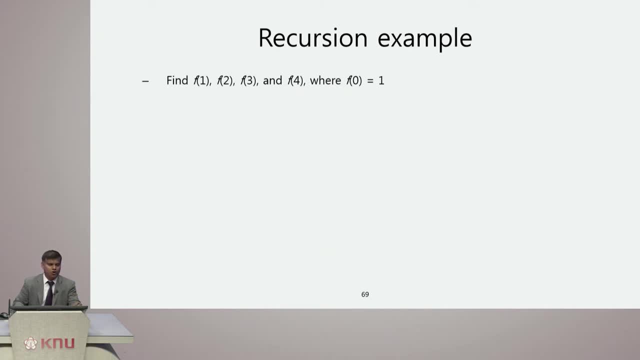 where f of 0 equals 1.. So we have this function, f of x, in which you have these things, are given to us. f of 0 is given by f of 1, f of 2,, 3, and 4.. 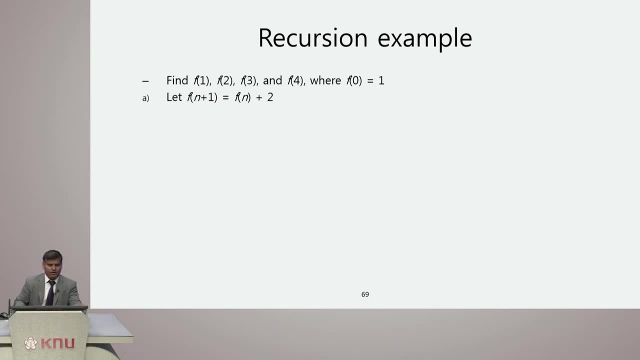 We have to find Here: let f of n plus 1 equals f of n plus 2.. So here is what is given to us. So with this we can find what is f of 1.. So we just write: f of 1 equals f of 0 plus 2.. 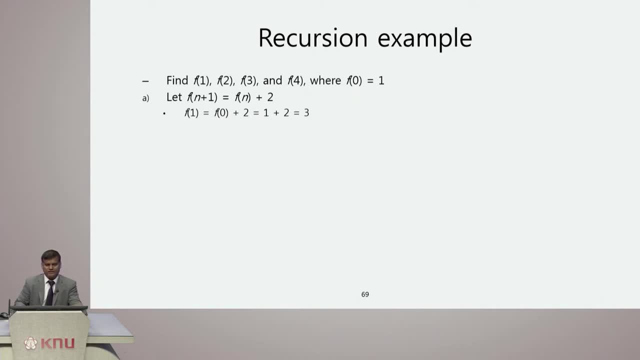 That is, in our case it's going to be 3.. The same way, if you want to find f of 2, then you're going to use f of 1 plus 2.. So that again is going to be 5, because you are using f of 1 over there. 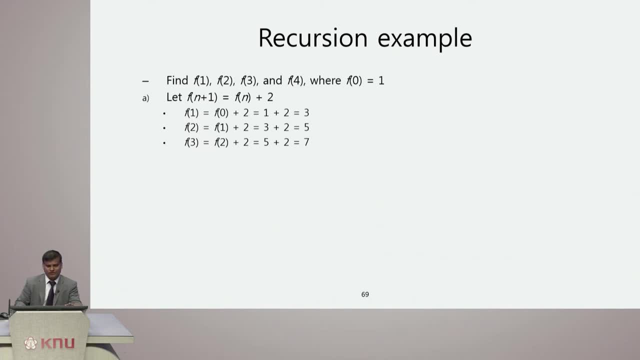 In the same way, f of 3 equals f of 2 plus 2.. So that is 5 plus 2.. That is 7.. And f of 4 equals f of 3 plus 2, because we just used this form right. 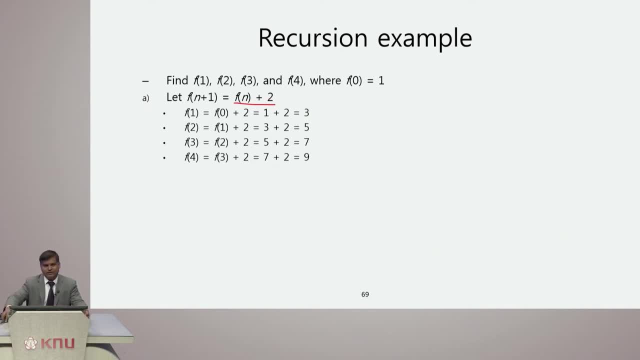 f of n plus 2.. So every time you just add 2 to it and you are getting a sequence of 2.. You are getting a sequence of 3,, 5,, 7, and 9.. And, of course, if you are asked to find f of 5,, f of 6, you would be able to find it. 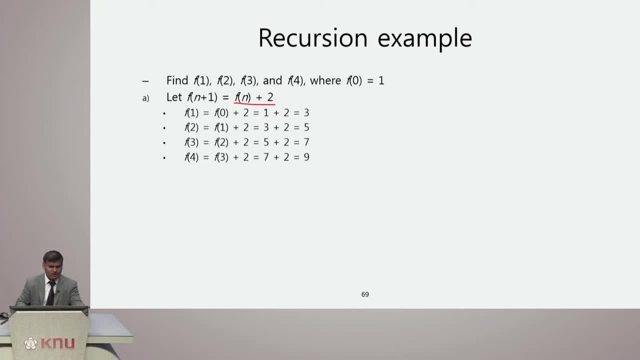 Yes, it's kind of calling this function to itself. That's the idea. For example, f of 1 calls f of 0, and f of 2 calls f of 1.. And f of 1 is nothing, but still the same function, right. 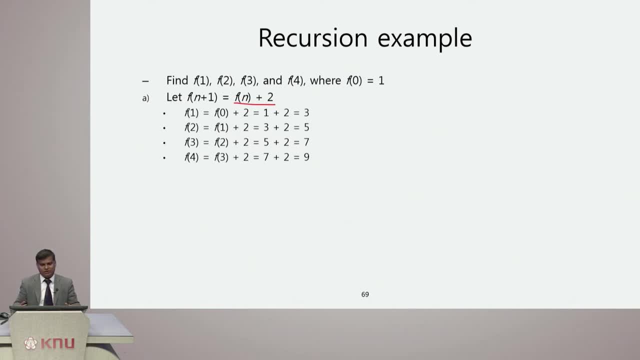 That f of n plus 2.. We are calling the same thing, We are calling the same idea, the same definition that has been defined for this function in this particular example. Let us consider another one, where f of n plus 1 equals 3 times f of n. 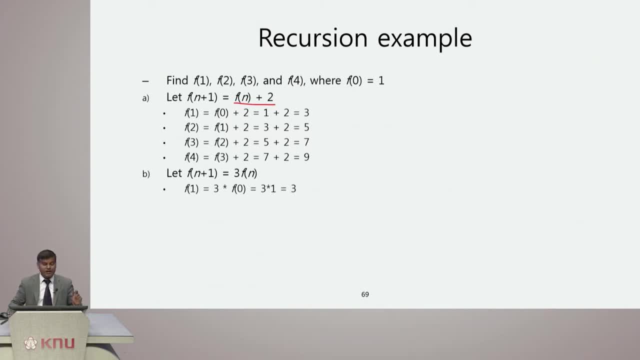 In this case, f of 1 equals 3 times f of 0. That is, 3 times 1.. Remember that f of 0 is given to be 1.. Do not forget that. So you know what is f of 0?. 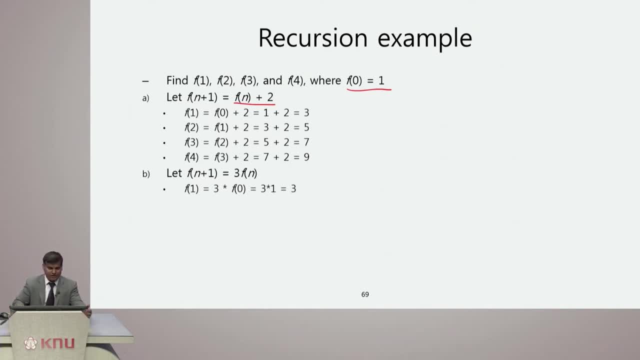 That is 1.. And f of 1 is 3 times that. And f of 2?? Yes, you can guess that f of 2 is f of 3 times f of 1.. That is 3 times 3.. 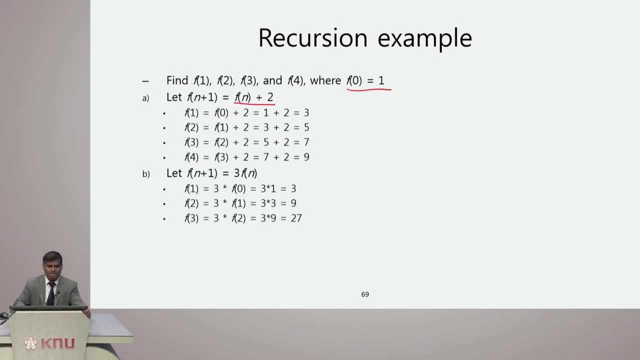 That is 9.. f of 3 is 3 times f of 2.. f of 4 is 3 times f of 3.. That is it. We are repeatedly calling the function to itself, And this is a very efficient way by which we can manipulate things. 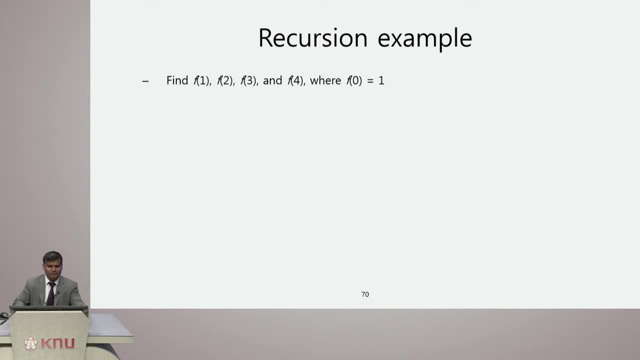 Recursion. more example. let us see here, Okay, The similar kind that you had here before. So now let us say that f of n plus 1 equals 2 power f of n. So let us consider this: f of 1 equals 2 power f of 0.. 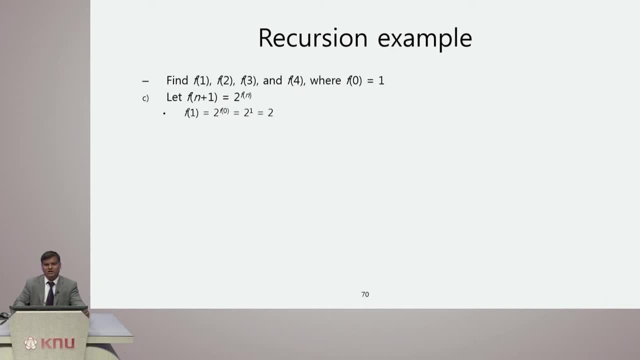 That is 2 power 1. That is equals 2.. And again f of 2 equals. we are calling f of 1 there. So 2 power, f of 1 equals 2 power, 2. That is 4.. 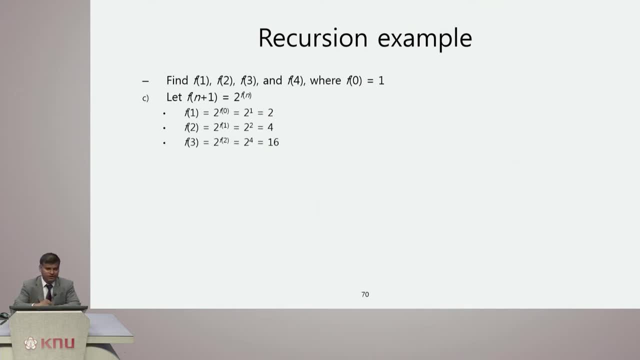 So if I repeat the same thing again- f of 3, you get the similar idea. f of 4, again you get a similar idea, You get a similar thought. So this is what a recursion means. We have another example here. 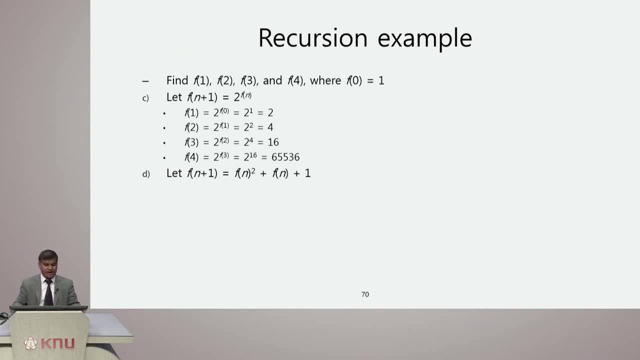 f of n plus 1 equals f of n square plus f of n plus 1.. So f of 0, again we can take that here It is given to be 1.. So f of 1 equals f of 0 square plus f of 0 plus 1.. 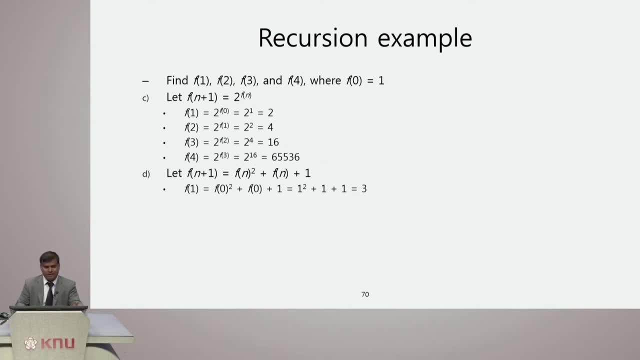 So that is 1 square plus 1 plus 1.. That is 3.. And if you want f of 2, then you have to use this value there. So f of 1 square plus f of 0 plus 1.. 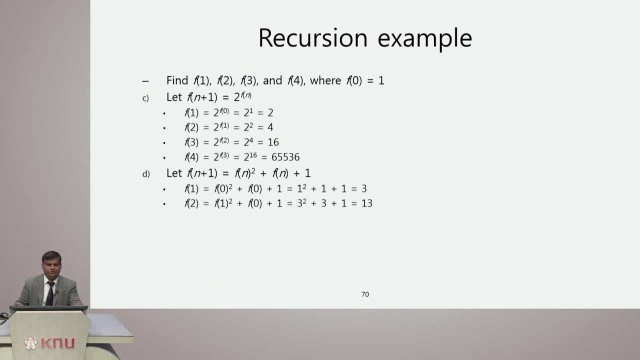 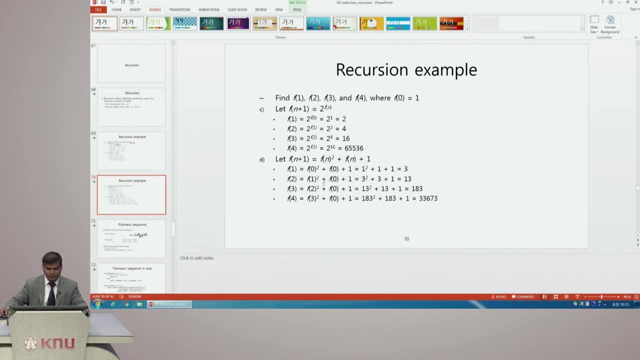 So in this case you have the values of- I suppose this has to be f of 1.. So we will just change this out. So in all these cases here we are supposed to have 1,, 2,, 3.. 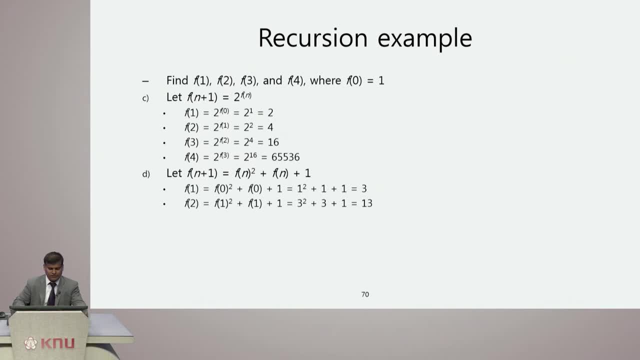 So that is right. So we are coming up with this f of 2, where we use f of 1. And for f of 3, we are using f of 2.. So that is right. So we are going to use f of 2.. 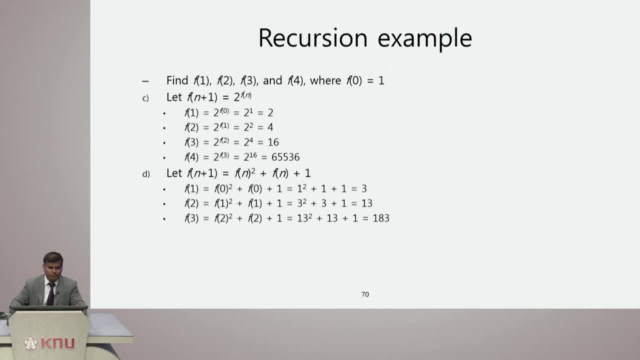 So for example, f of 3 equals f of 2 square plus f of 2 plus 1.. That is 13 square plus 13 plus 1.. That is 183.. And f of 4 equals f of 3 square plus f of 3 plus 1.. 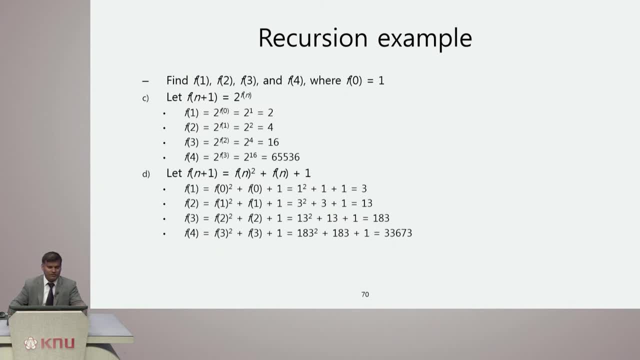 That is 183 square plus 183 plus 1.. That is 3,, 3,, 6,, 7, 3.. So that is it. We have come across four examples of regression Fibonacci sequence. even we can represent this Fibonacci sequence in terms of a recursive 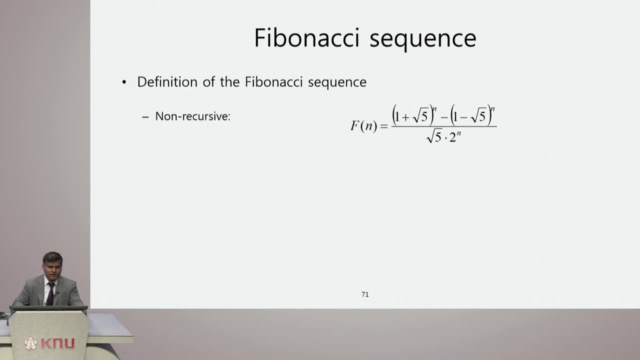 function. So, as we have seen this one formula earlier when we talked about sequences- but this is a non-recursive function- But this one, this f of n equals f of n minus 1 plus f of n minus 2, this is a recursive. 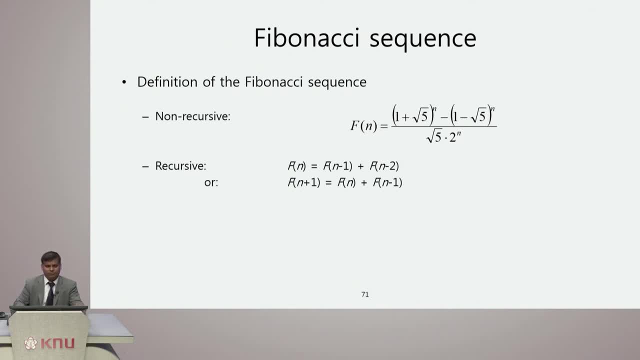 function. So you could also represent: by means of f of n plus 1 equals f of n plus f of n minus 1.. So what is the main thing here is that we have to define the base case, because you know that Fibonacci series starts with 1,, 1, and then goes on to add the previous values. 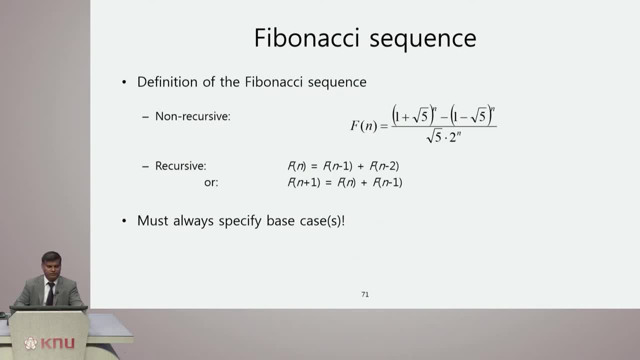 like 1 plus 2, 3, 3 plus 2, 5.. So the base case here f of 1 is 1 and f of 2 is 1.. So the first two functions are 1 and 1.. 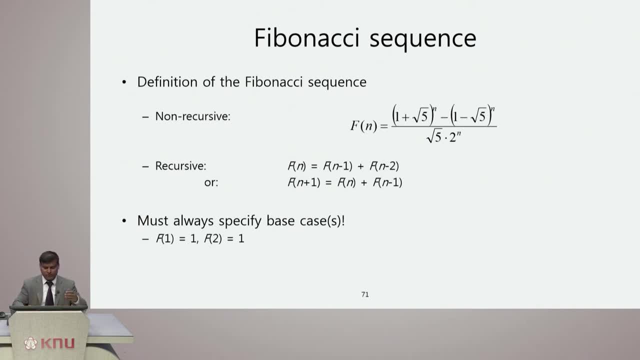 Starting from 3 onwards, you are going to change. that is 1 plus 1 is 2, that is your f of 3.. So the base case here is f of 1 and f of 2 is given to be 1.. 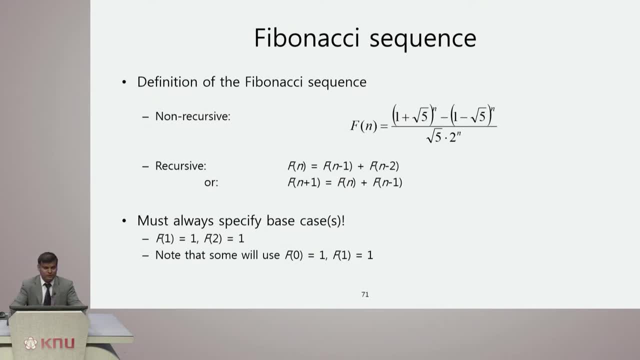 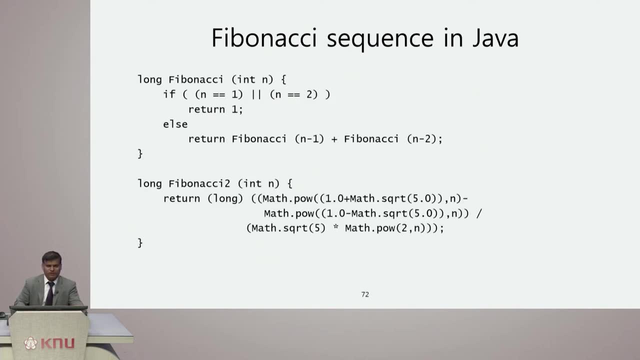 So sometimes people use f of 0 and f of 1 here. It depends. So anyway, the basic thought is here to use the base case properly. So here is a simple code for Fibonacci sequence in terms of Java programming. 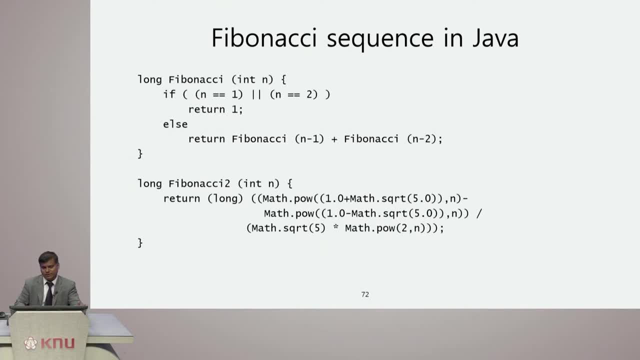 So you can have a look at it. If you are familiar with C++ or Python, maybe the things might be different And in fact there are some packages available for if you are using Python or other tools like MATLAB and so on. 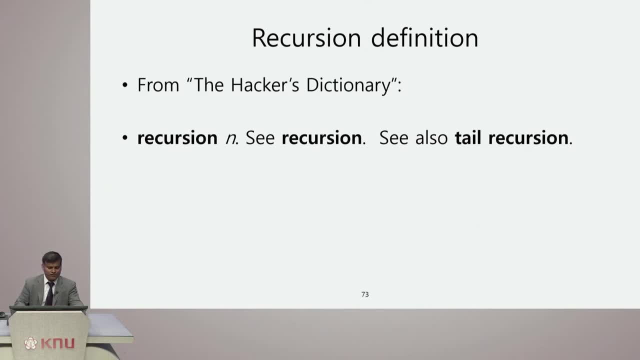 So I will skip this off. There are a few definitions in case of recursion, recursion, recursions, tail recursions and recursive, And in fact we have also have things like transversive functions. So this is an example of a bad recursive definition. 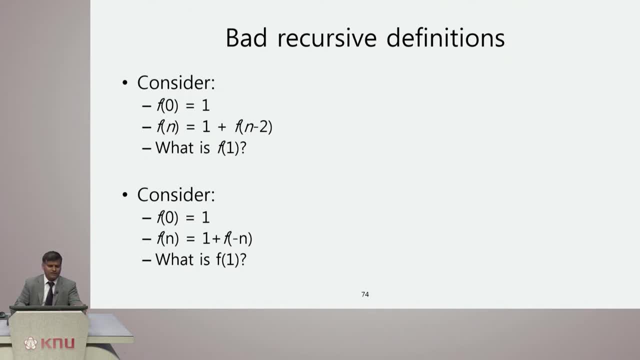 You can see, like you can define: f of 0 is 1.. f of n is 1 plus f of n minus 2.. So in this case you would be like just try to find f of 1.. So this is like it goes. it takes you to some negative value and then you get struck. 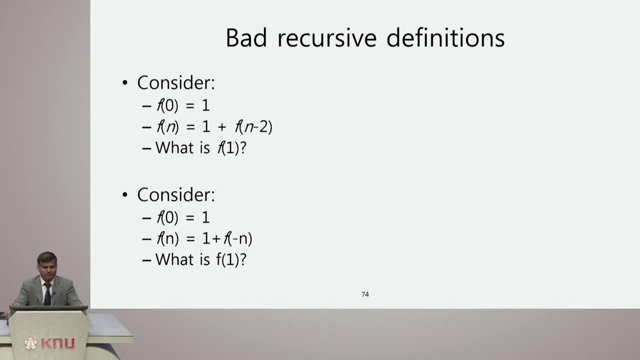 with that? Yes, that might happen. The same way if you consider the second one: f of 0 equals 1, f of n equals 1 plus f of minus n. Again, it takes us to some negative values there. So anyway, basically, if you really want to define a function for negative integers, 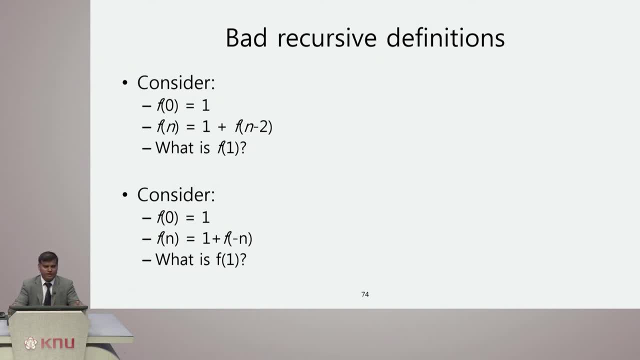 or some other values of real values. you might be specifying it clearly. You have to define clearly. You have to also define the base case clearly: where to start and when to finish, based on the application. Okay, So defining sets via recursion. 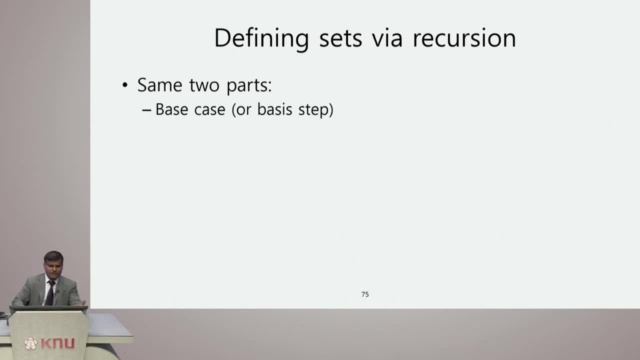 So, for example, we just use the same two parts, like the base case or the basic basis step, recursive step. If we recall the induction method, we use the base case, then we use the inductive induction proof and then the induction step we use right. 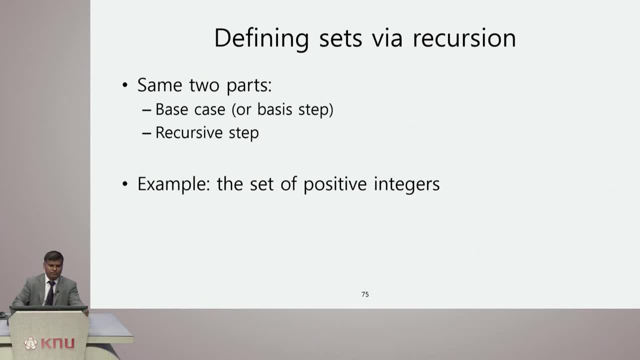 But here we use base case and the recursive step. So let us say this example: the set of positive integers, say 1, is an element of s, and recursive step is: if x is an element of s, then x plus 1 is also an element of x. 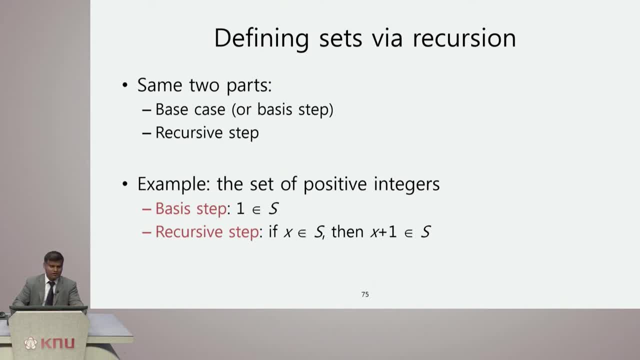 Does it sound familiar? Yeah, that is similar to the induction principle that we used to use. right, If you assume that for a certain value, if this is true, then we have to prove that for the next value, that is x plus 1, it has to be true. 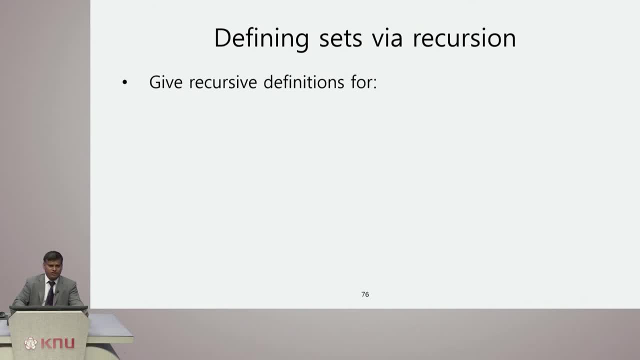 So, defining sets via recursion, we have this say, for example: set of odd positive integers given 1 is an element of s, and if x is an element of s, then we have to say x plus 1 is an element of s. 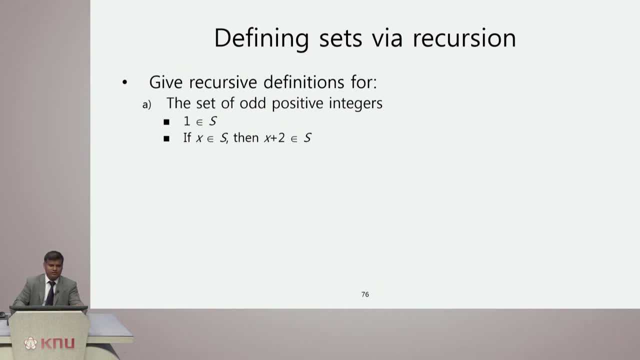 Then we have to say, or we have to prove that x plus 2 is an element of s. So that is one other example. here we have The set of positive integer powers of 3,. 3 is this element of s. and then here you have. 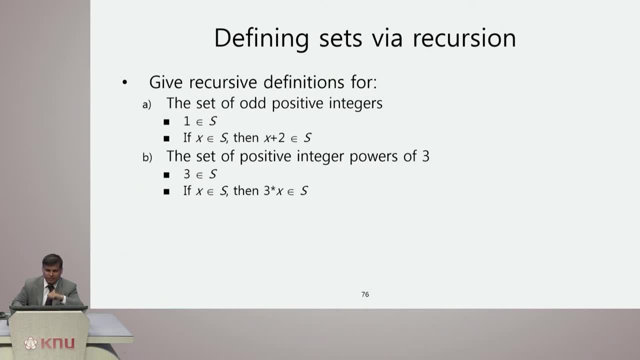 x is an element of s, then 3 times x is an element of s For set of polynomial, For set of polynomials, For set of polynomials In terms of powers, Set of polynomials with integer coefficient. So 0 is an element of s. then if p of x is element of s, then p of x plus c times x power. 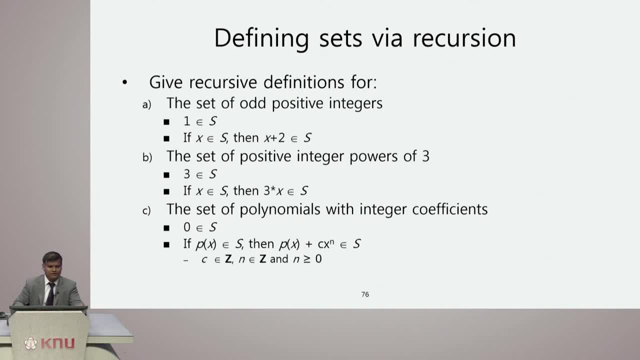 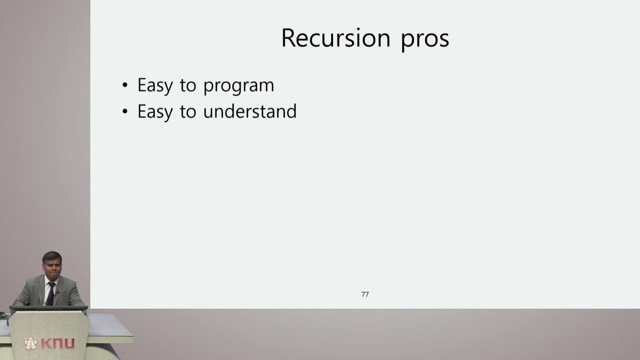 n is an element of s. So here some thoughts like: c is element of z, z here indicates the integers, and n is an element of z. then and n is greater than or equal to 0.. Okay, recursion pros. easy to program, easy to understand. 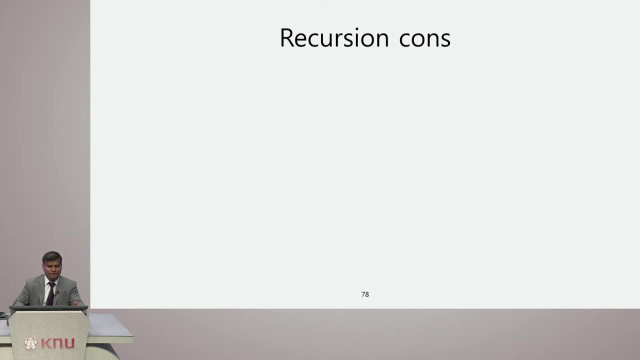 Of course that is interesting, but we should be careful. I will come back to this. Well, we see why I said we should be careful, because here it comes: recursion cons. Okay, consider the recursive Fibonacci generator. Suppose you are, Suppose you are writing a program to generate a Fibonacci sequence. 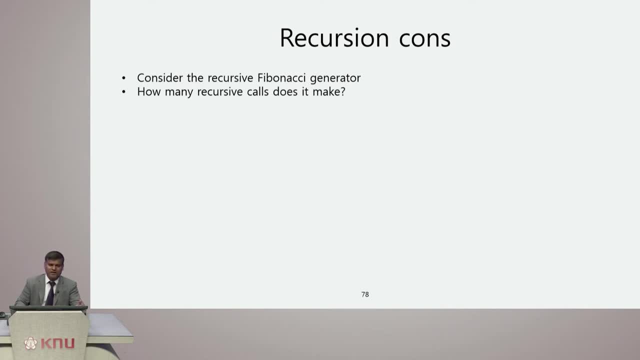 How many recursive calls does it make? Let us say f of 1 equals 1, f of 2 is 1.. We know these two are the base case, right, We have 1 and 1.. Starting from the third one, we are going to use the formula. 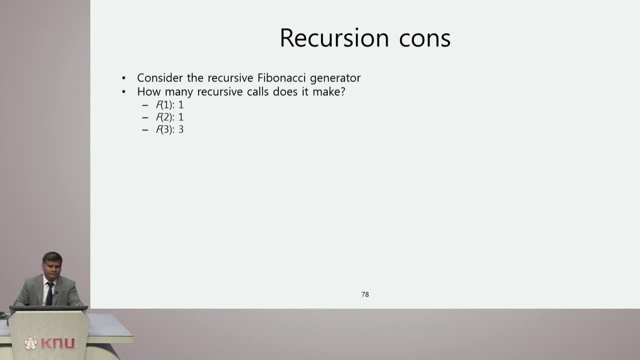 So f of 3 is 3.. It is supposed to be Okay. we have 1, 1 and 2, 3, 5, supposed to be 8.. f of 10 is 109.. And we have f of 20 is 13529.. 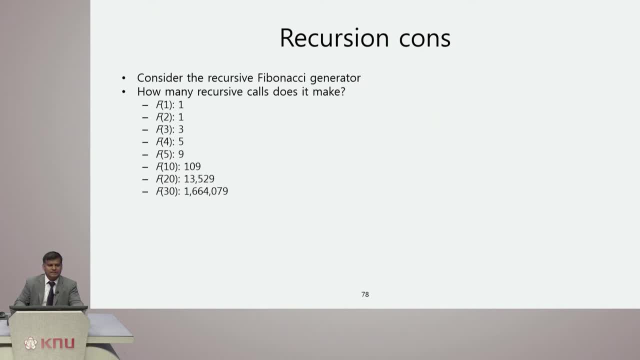 f of 30 is 1664079.. Then here comes f of 40,, 204,, 204,, 668, 309.. So well, here comes the next one, f of 50.. That is 25, 172,, 538, 049.. 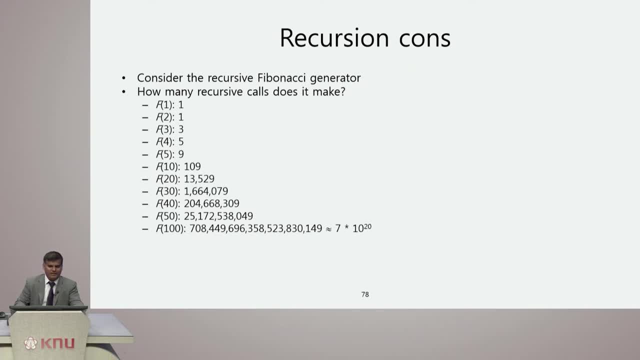 Well, this f of 100. That is too big for me. Well, you could consider having approximated to 7 times 10 power 20.. Well, what is wrong with this At 1 billion recursive calls per second, if your computer is quite fast enough. 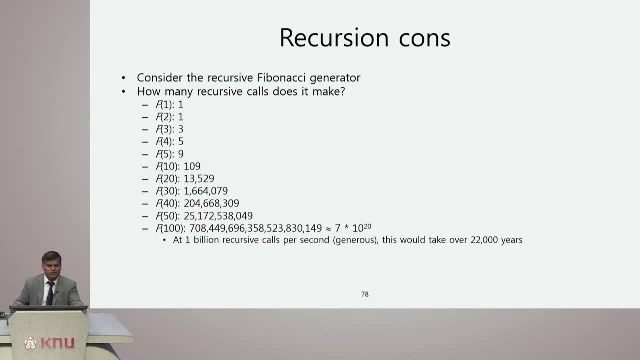 it would take over 22,000 years. Well, that is where we have to be careful when it comes to recursion. So at times the recursion also can lead you to some deadlock conditions, But that would also take over 10 power, 12 GB of memory. 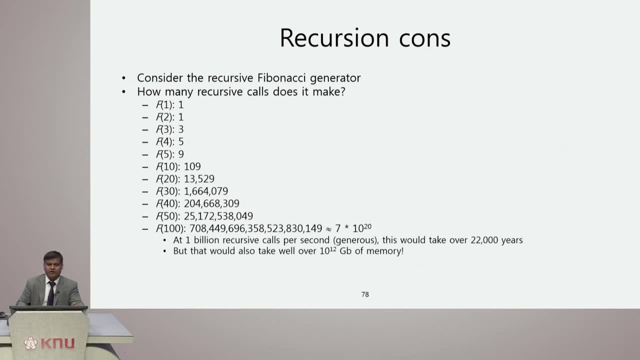 That is huge, very huge. Well, this is one of the drawbacks that you have in case of recursion functions. Let me briefly tell you one more place where we should be very careful when we are considering the recursion, For example, in case of a recursive call. 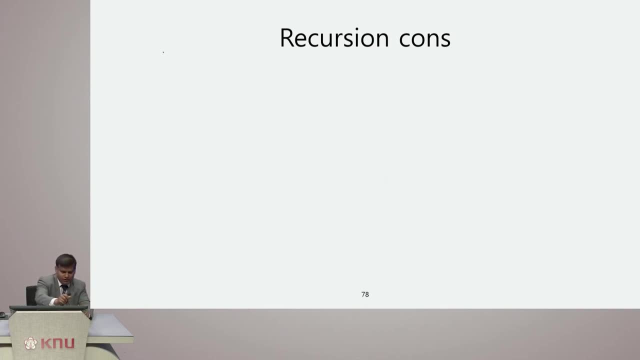 suppose you are writing your program and then you have function say, function f, Fun 1.. Say, you have here this Fun 1 is here. And then you have another function, Say fun 2 is here. And while you are going through these functions, 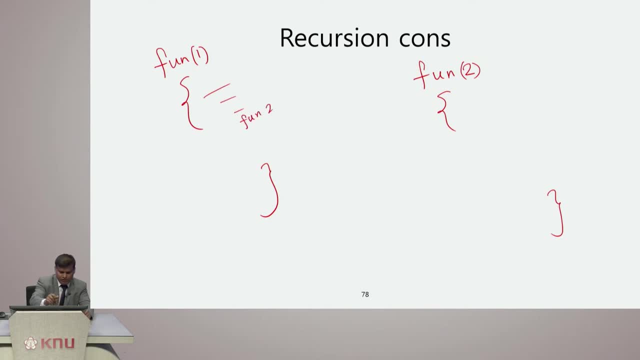 you are calling fun 2 here, And when the fun 2 or function 2 is called, the command goes over this place and it starts to execute. And what you are doing here is you are calling function 1.. So when you call function 1, what happens? 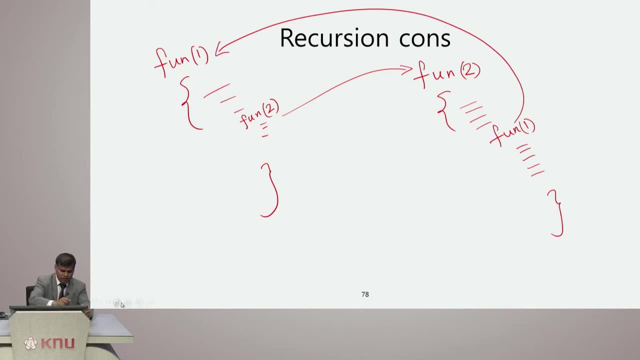 Again, the call goes back to this position. So what is happening here? Function 1 calls function 2. And function 2 calls function 1. So this is what we call a deadlock condition. So the system gets struck with this. 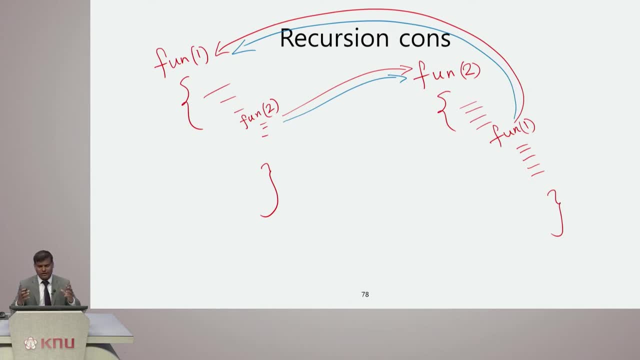 and it cannot be able to get out of this kind of recursive calls. So that is where we have to be careful in order to avoid such conditions. In terms of electronics, if you are working with microcontrollers at times, we do have assembly. 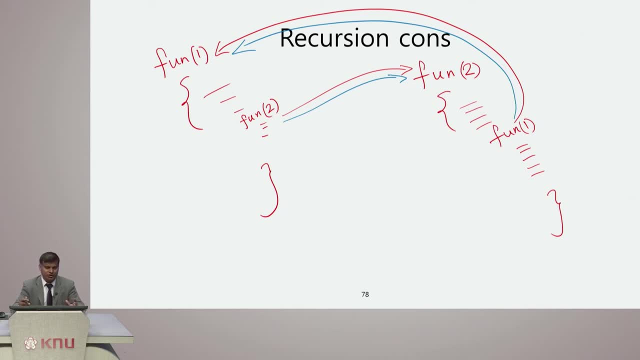 We do have assembly programming by using recursive calls, And to avoid such things, people use a timer called watchdog timer. In the same way, we can also use a simple timer mechanism, or we can just wait for a while, and if it does not come out of this function. 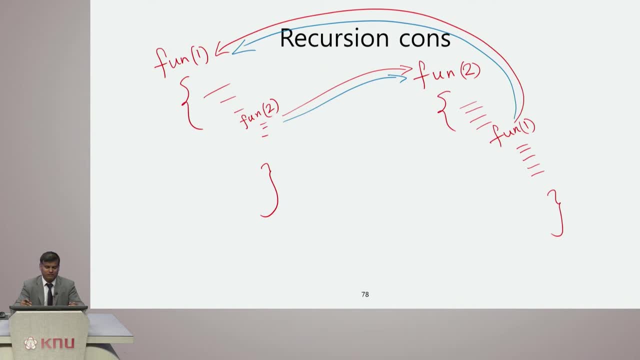 we try to quit this particular skip, this particular function. We can code such a way, Or, in other words, while these functions are going through this loop of calling one another, if a certain threshold is met, you should be able to come out either while you are here or while you are here. 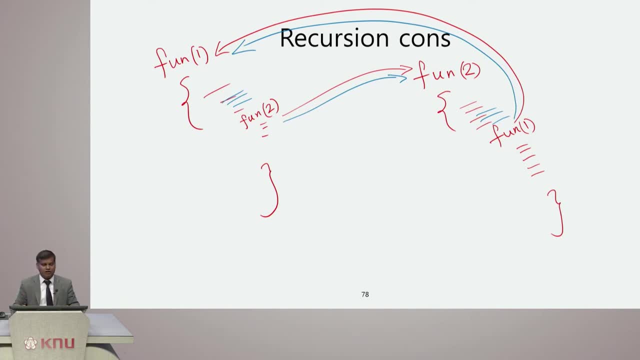 You should be able to come out of this deadlock state. Well, that is another problem that you can think of when you go on for programming. Okay, So let us move on with this recursive part. Recursion versus induction. Consider the recursive definition for factorial. 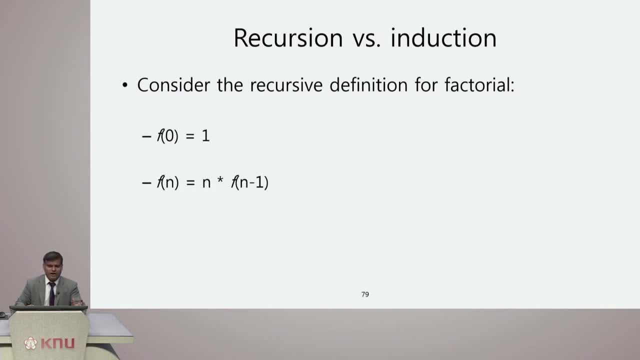 Well, f of 0 is 1.. f of n equals n times f of n minus 1.. So you have this f of 0 equals 1 as the base case, And here this n times f of n minus 1 is going to be your inductive step. 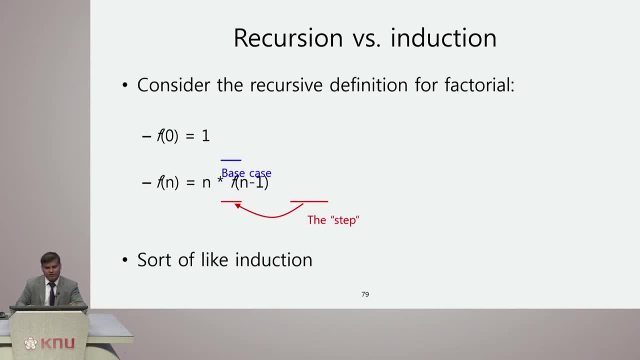 So it is kind of, this is a sort of induction. So you have base case and you have this inductive step In this recursion part. we call it as recursive step. Yeah, that is very similar to induction that we have talked about. 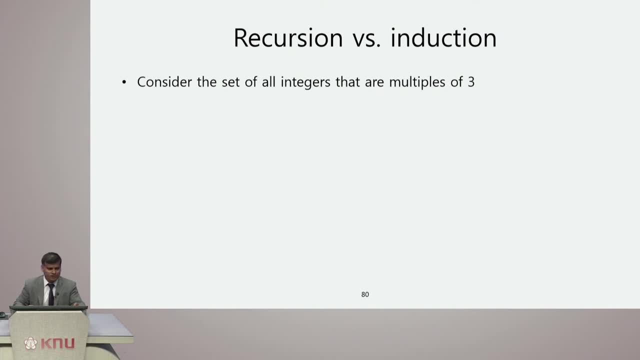 Consider the set of all integers that are multiple of 3.. You have this set given to you with 3,, 6,, 9,, 12, and 15, and so on. So we say that, well, x equals 3 times k. 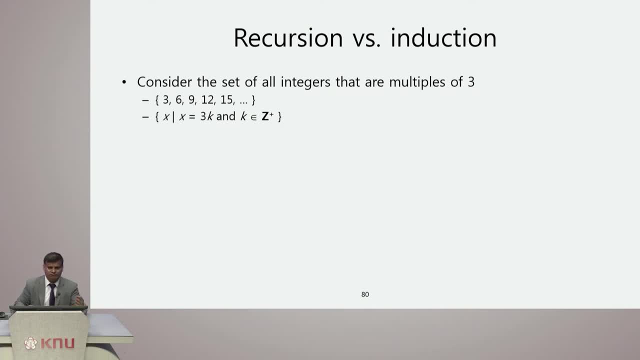 and k is an element of z, positive, that is, positive integer. So by recursive definition, the basic or basis step that you have here is: 3 is an element of s And recursive step is if x is an element of s and y is an element of s. 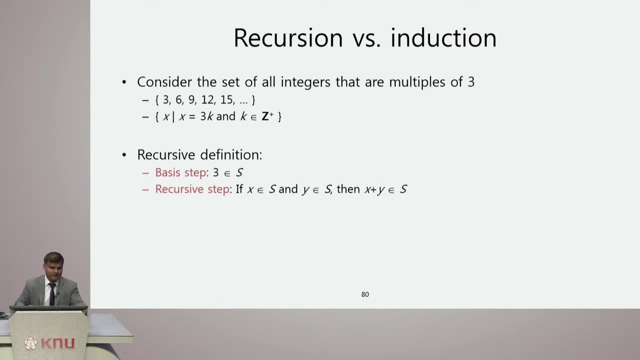 then x plus y is an element of s. So that is one example that we have seen. Let us see recursion versus induction with another proof, proof via induction Proof that s contains all integers that are divisible by 3.. So let a be the set of all integer divisible by a, by 3,. 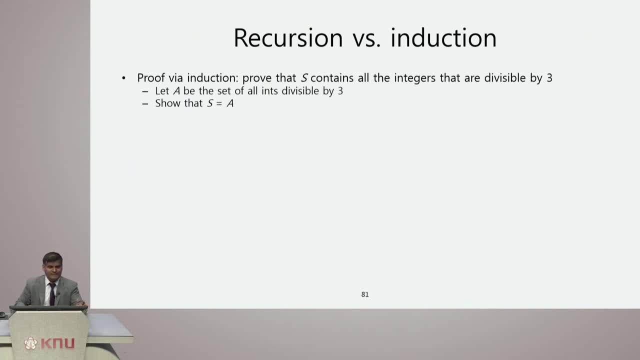 and show that s equals a. So we have two parts. One is to show s is a subset of a. The other one is a is a subset of s. Got it? I repeat this part again. We are asked to prove that s contains all integers that are divisible by 3.. 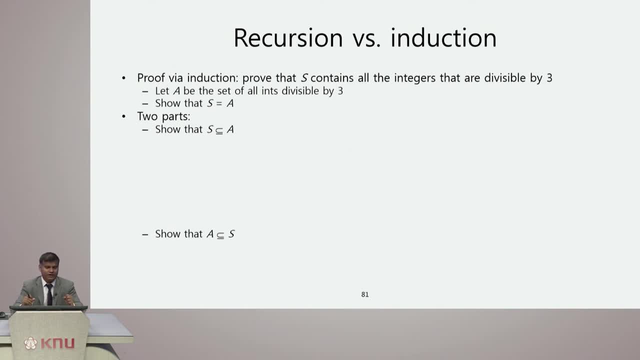 And we are saying: let a be the set of all integers divisible by 3.. So you have the set a, which has all the integers that is divisible by 3.. So we are asked to show or prove s equals a. 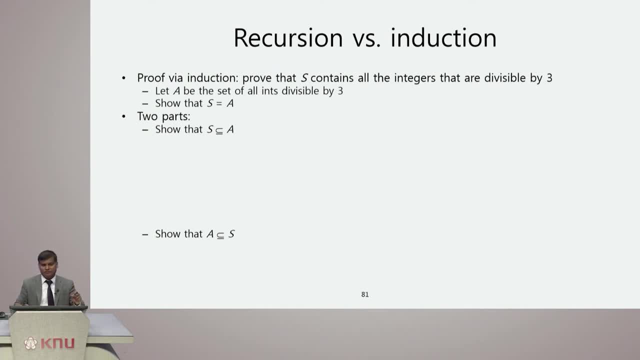 To show that. there are two parts you can prove it. One is: you can show that s is a subset of a and a is a subset of s. Well, let us say: p of n equals 3 n. 3 n is an element of s. 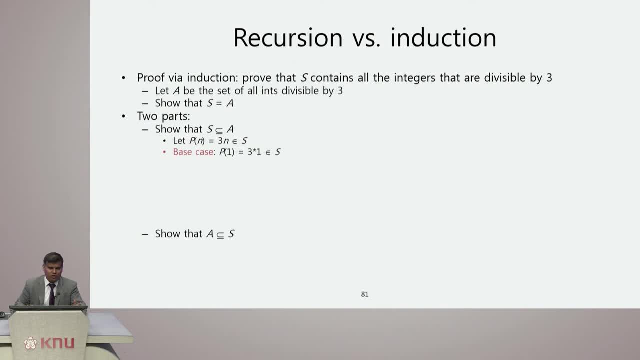 And then you have the base case: p of 1 equals 3 times 1, which is element of s. So by basis step of this recursive definition, we are using this base case And, with inductive hypothesis, we assume that p of k equals 3 times k is an element of s. 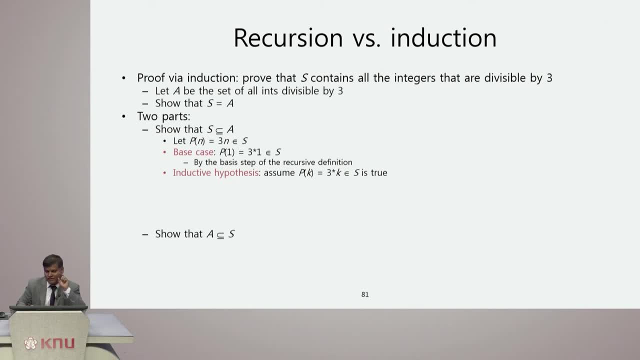 That is the inductive hypothesis. So we assume that that is true. And what is our next step? We are going to say the inductive step for p of k plus 1, we have to prove that for p of k plus 1,. 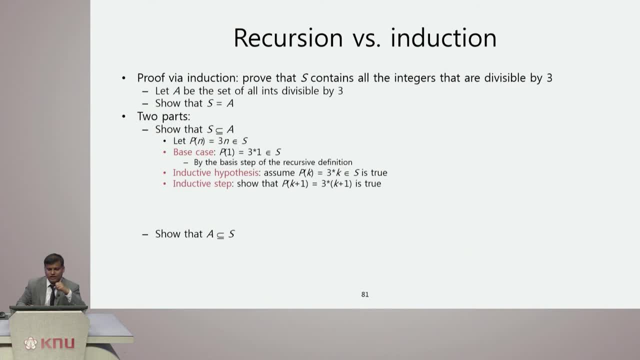 it has to be true. So p of k plus 1 equals 3 times k plus 1, is true. So let us see here: 3 times k plus 1 equals 3k plus 3.. So 3k is an element of s by inductive hypothesis. 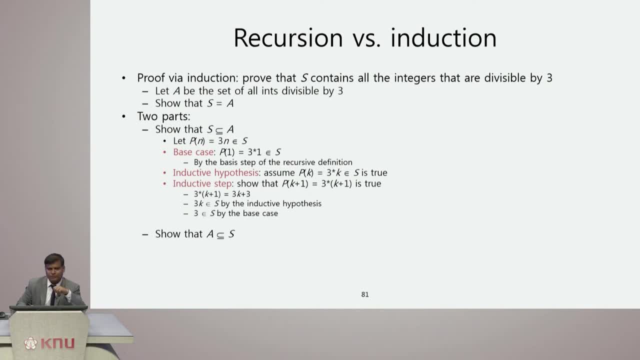 that we have seen earlier. Therefore we have: 3 is an element of s by the base case. We have already seen that one as well. So thus 3k plus 3 is an element of s by recursive definition. So by means of, we started with the inductive proof. 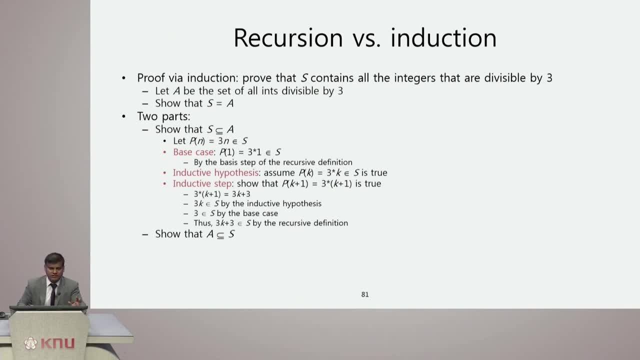 but we have concluded with the recursive definition by showing that s is a subset of a. Now consider this similar step. use it, for a is a subset of s. So you can try, try out by yourself which has the similar sets. 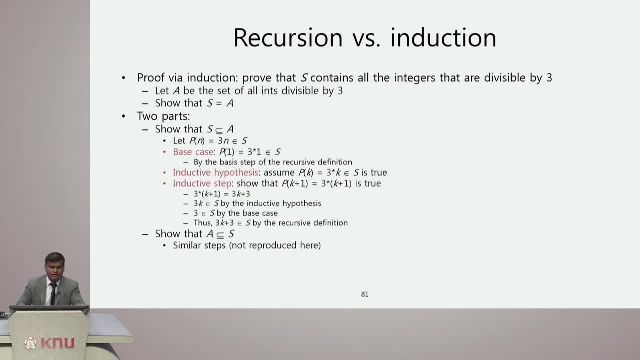 So, basically, just we have to. we have proved that s contains all the integers that are divisible by 3, because we used another set, a, and we assume that a also has a set of all integer divisible by 3, and then that is it. 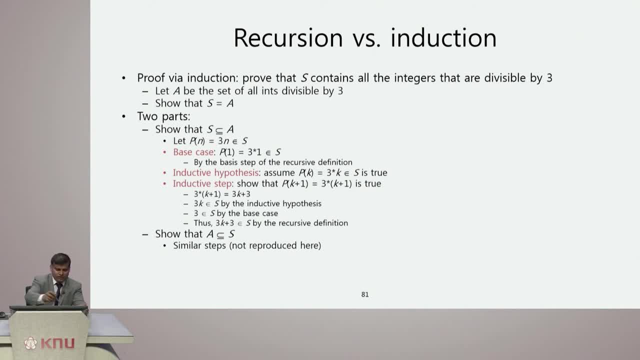 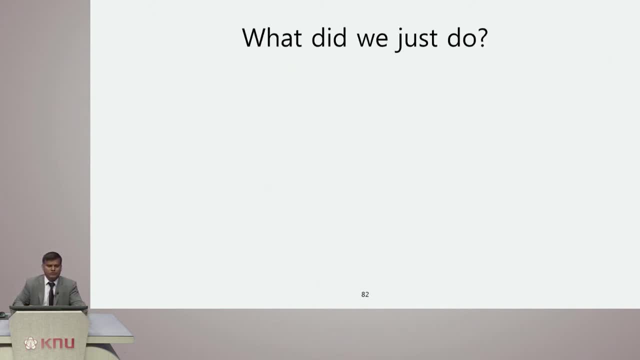 we proved it right And we showed that s is equal to a. So what we just do is the way we express this recursive form of proof. So let us see: We showed the base case to be true. We proved that is true. 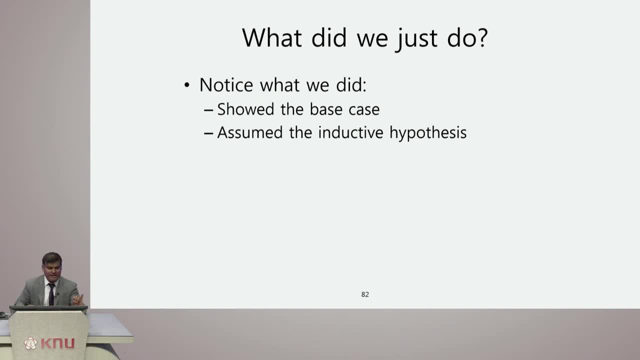 Then we assume the inductive hypothesis as before. After assuming the inductive hypothesis, our next term is to prove the inductive step. Yeah, We proved the inductive step. So for inductive step, we showed that each of the parts were in s. 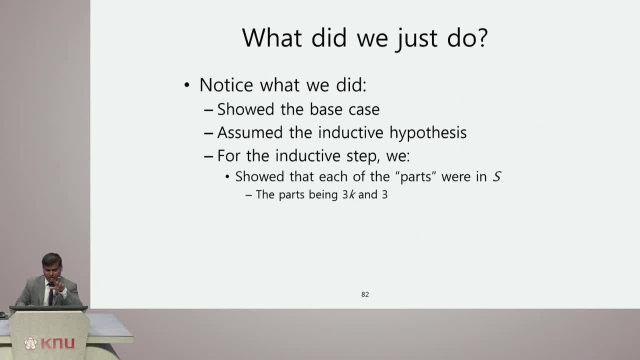 the parts being 3k and 3.. Here are two parts that were there in s, and 3k has been proved in inductive. 3k is one of the assumptions, that is, 3k is our inductive hypothesis or assumption. 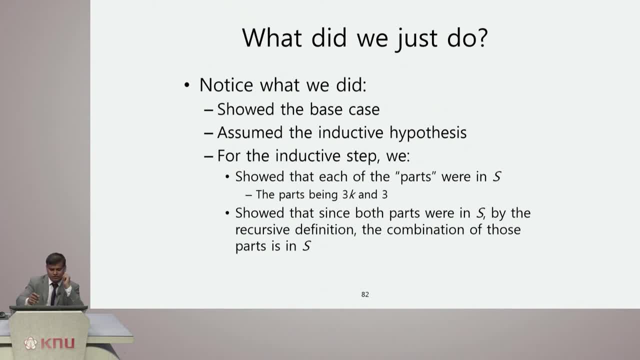 and 3 is a part of the base case. So these are the two parts we had. Yeah, So we showed that both parts were in s. We showed that 3k as well as 3, both are in s. 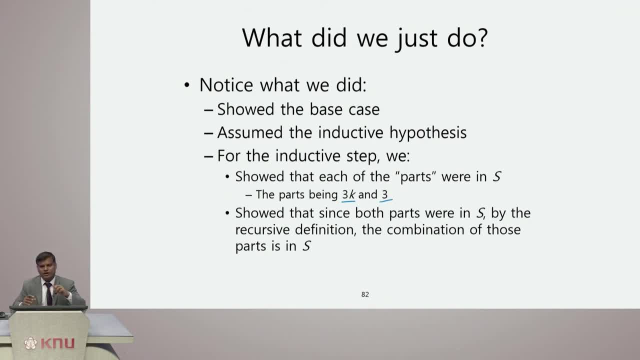 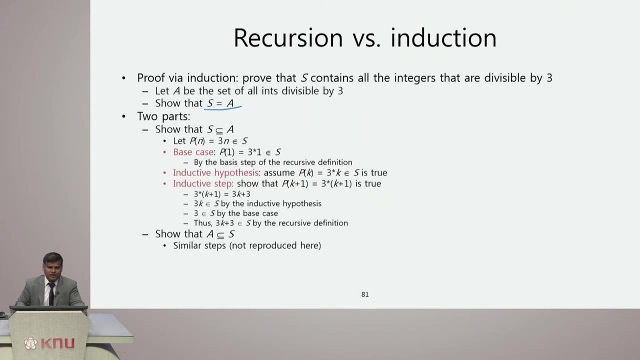 By the recursive definition. the combination of those parts is in s: Yeah, We had this, both parts, So that is, if you want to quickly look at what is went through, you can just have a look at this and you will clearly see that. 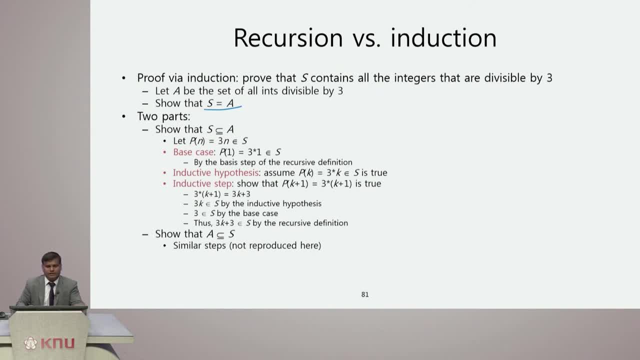 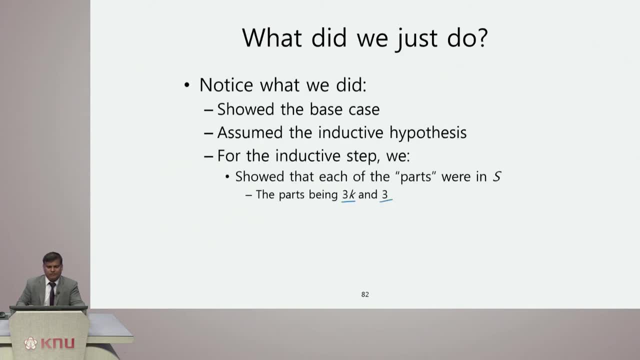 we have proved it using the recursive definition. Okay, So this is what we have done, And this is also called structural induction. So when you prove things by means of a recursive definition, we can call that kind of proof as structural induction. 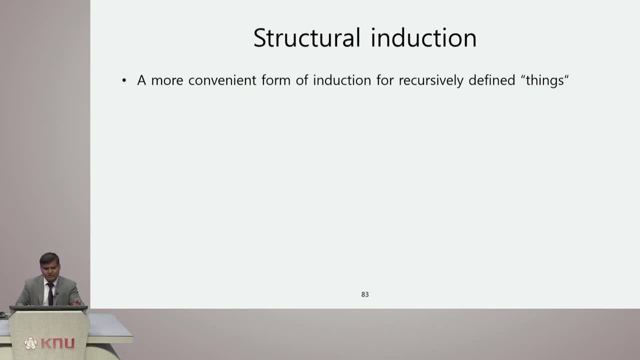 So, talking about the structural induction, so this is one of the convenient form of induction for recursively defining things, When used in conjunction with recursive definition. we have three parts: The basis step- show that the result holds for elements in basis step. 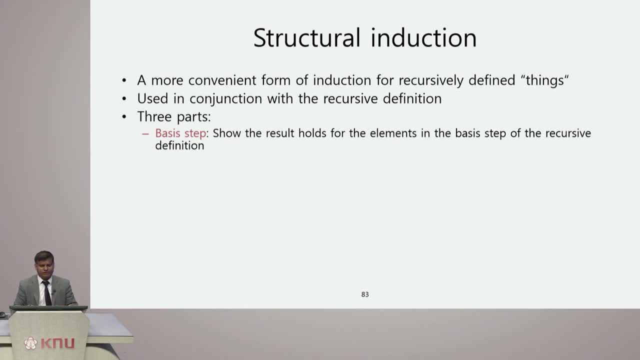 for recursive definition. So that is your base case. Then comes the inductive hypothesis. You assume that the statement is true for some existing element, for some element It is true. It is same as the inductive proof that we have seen earlier. 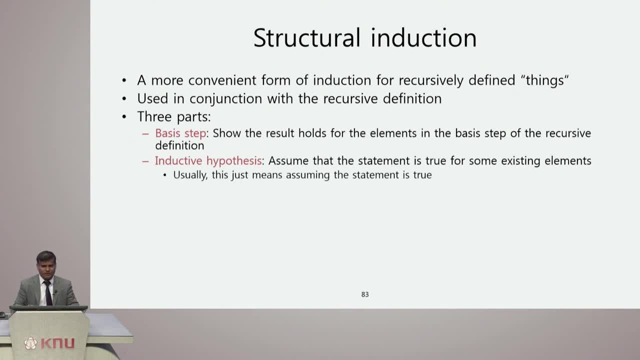 the proof by induction. The third step is your recursive step. But in inductive hypothesis we usually this just means assuming the statement is true. So for some existing case we say that the statement is true And for recursive step. 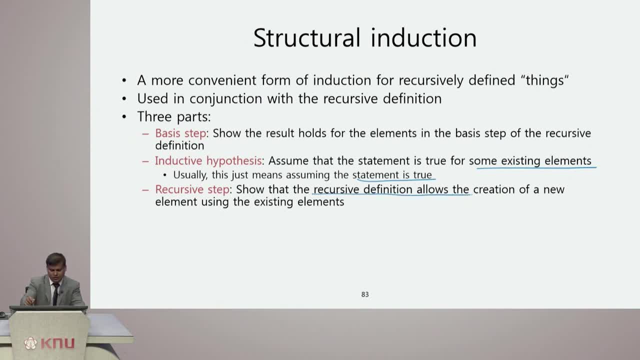 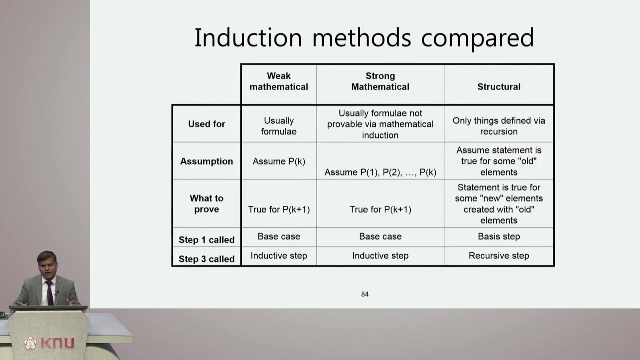 show that the recursive definition allows the creation of new elements using the existing elements. So it allows the creation of new elements using the existing elements. That is the recursion right. So here is the basic outline of what you have for this induction methods. 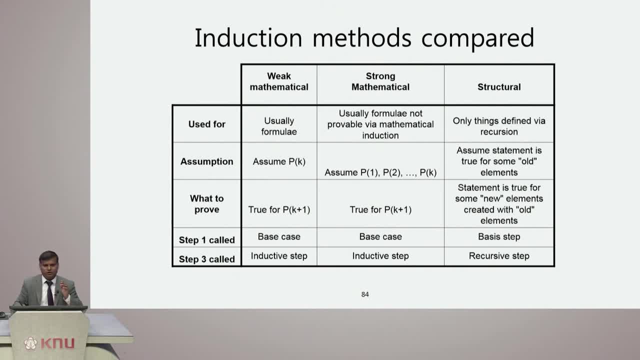 You can see we talked about the weak mathematical induction. strong mathematical induction, structural structural induction, And weak mathematical induction is used for, usually for basic formulas, And the basic assumption is that assume p of k, we assume p of k and then we have to prove p of k plus. 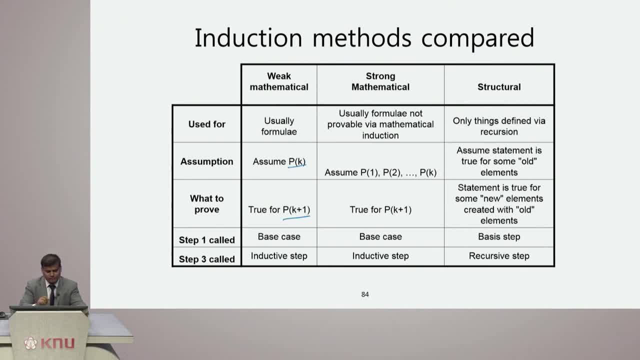 we have to prove p of k plus 1 is true. So initially we have the base case and then the step 3 is inductive step. So for the strong mathematical induction usually formulate not provable via mathematical induction. So it is very hard to prove using the basic mathematical induction. 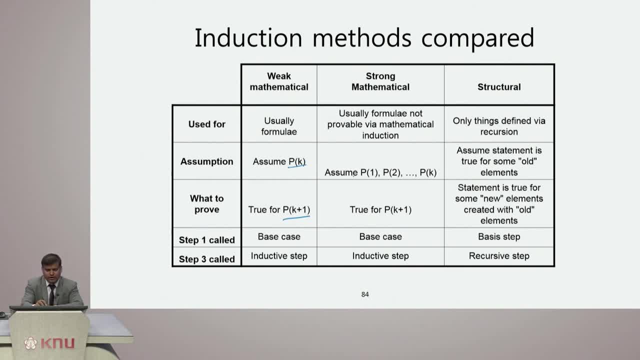 So here we are going to assume that p of 1, p of 2 till p of k, all are true. Then we have to prove: for p of k plus 1 is true, The same base case and inductive step is applied. 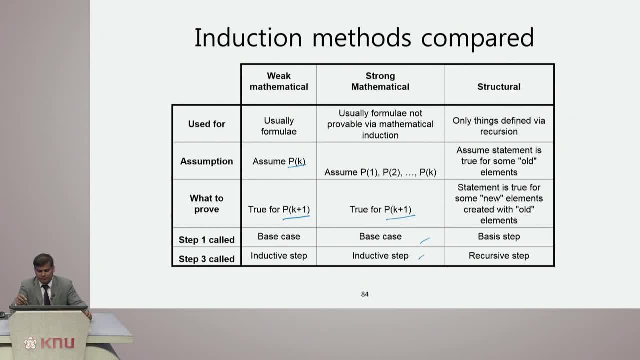 For structural induction. so only thing defined via recursion we go for the structural induction. So we assume that is true for some old element or some elements that are existing, some elements that are existing As we have seen here earlier, some existing element. 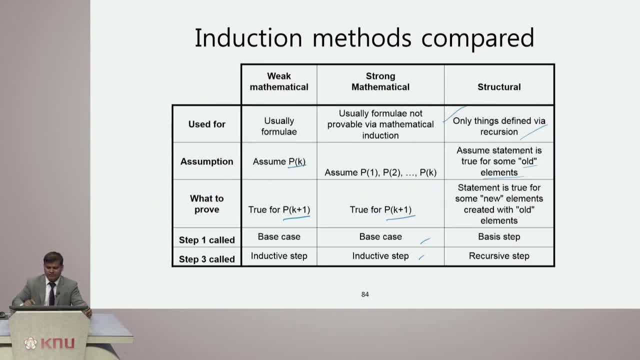 it has to be true for some existing element, And then the statement is true for a new element, a new element that exists That you are able to create using the recursion. So it is true for the new element, elements created with the old elements. 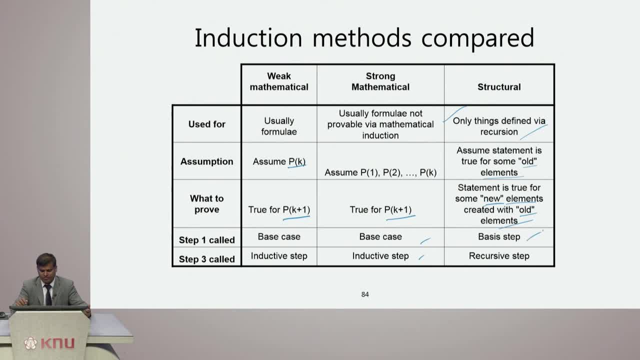 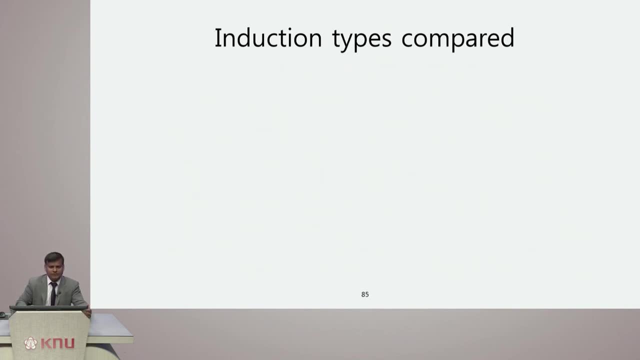 So that is what we have to prove- and uses basis step and recursive step. So basis step is similar to the Dof base case that we have for mathematical induction. Let us go further and see some induction types compared. So f of n is less than. 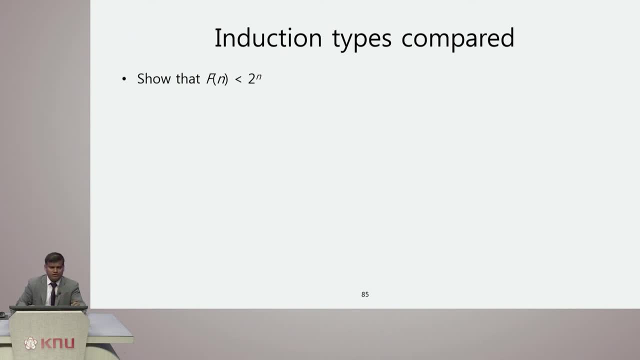 2 power n. So we have to prove this one. So where f of n is the nth Fibonacci number, actually f of n is less than 2 power 0.7 times n. But we do not have to prove that here. 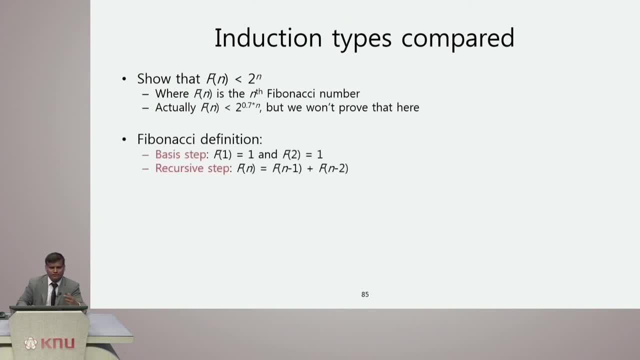 We do not really have to prove this. So, by means of definition of this Fibonacci, we know that f of the base case is f of 1 and f of 2, both are 1.. And then the recursive step. we have the same formula. 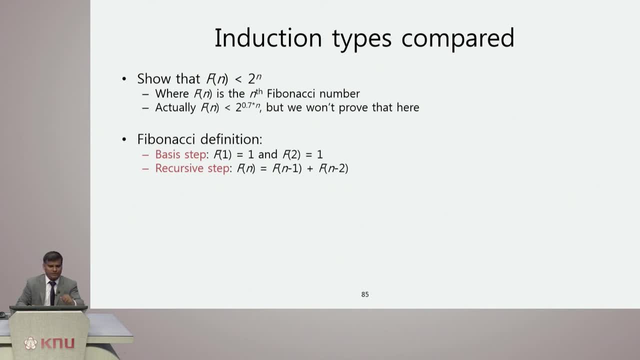 f of n equals f of n minus 1, plus f of n minus 2.. So the base case or the basis step, we show that it is true, because we have to show at first. this is: this is very essential. 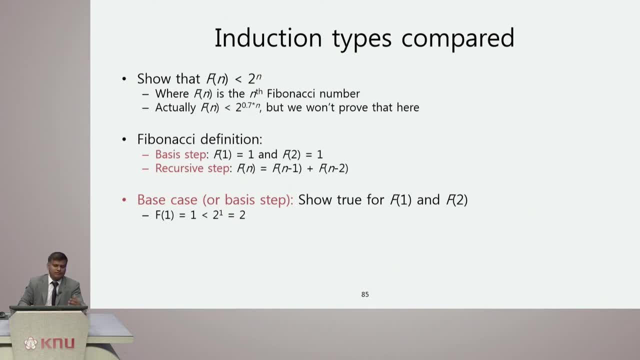 So f of 1 equals f of. I mean f of 1 equals 1, less than 2, power 1, that is 2.. f of 2 equals 1, less than 2, power 2, that is 4.. 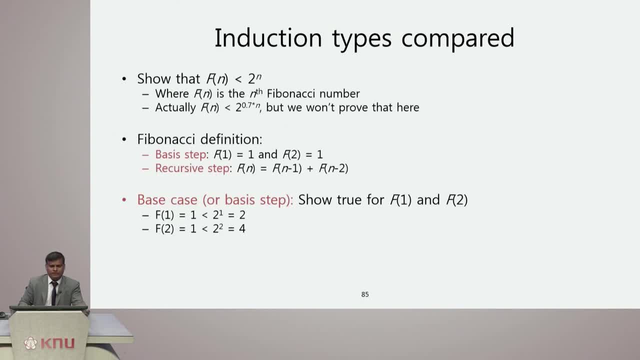 So here you can see, there is some, some values that you have come up with in which it does not really shows the actual base cases. true for the given, for the given function. So if we talk about a function, 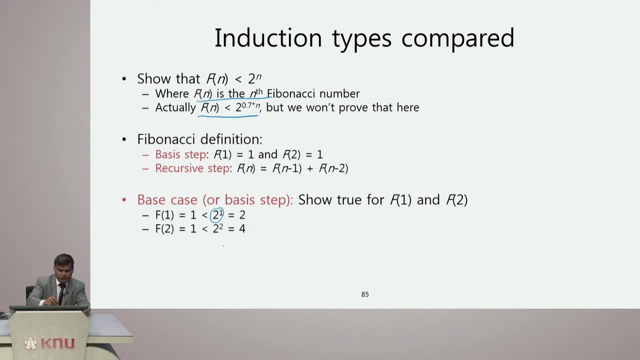 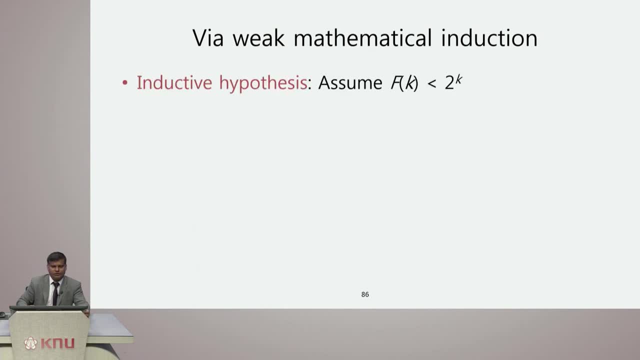 that is, of 2 power 2 power n, then this is how it looks like. So why a weak mathematical induction? Suppose, if you have f of k is less than 2 power k, then inductive step is: 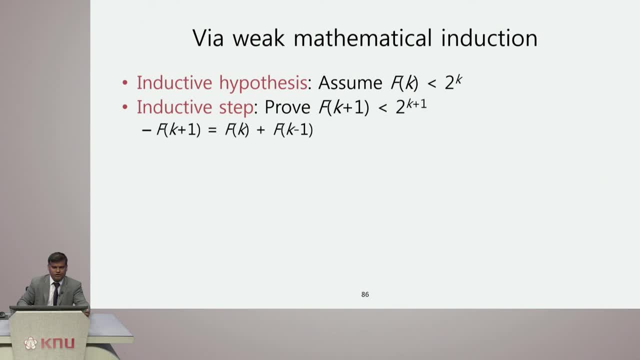 f of k plus 1 is less than 2 power k plus 1.. So f of k plus 1 equals f of k plus f of k minus 1.. In that case we know that f of k is less than 2 power k. 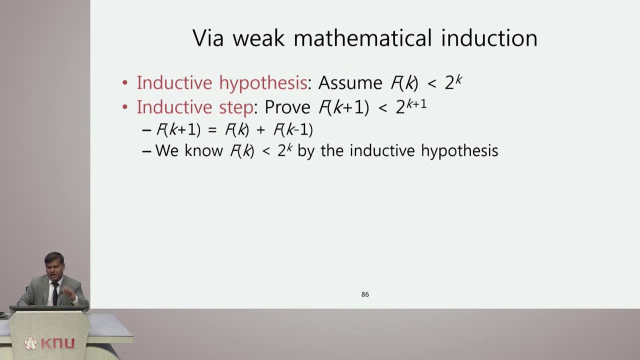 by inductive hypothesis. So that is an assumption that you have, And each term is less than the next term. Therefore, f of k is greater than f of k minus 1.. So, with this thought in mind, 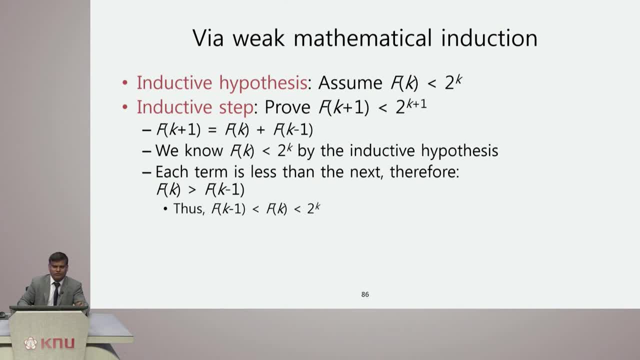 we can say that f of k minus 1 is less than f of k less than 2 power k. So therefore f of k plus 1 equals f of k plus f of k minus 1, less than 2 power k. 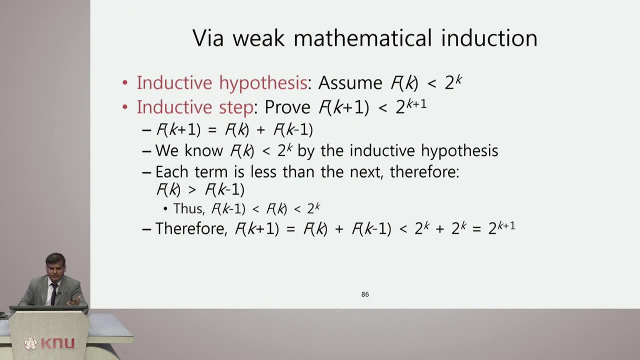 plus 2 power k, that is equals 2 power k plus 1.. So that is how it has been proven. So we are having this inductive hypothesis in which we have to prove it. 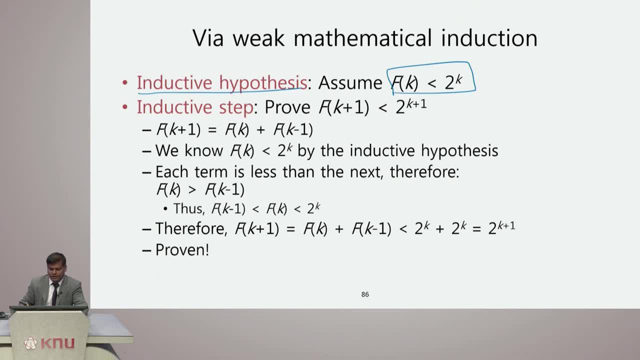 for a particular value, k Initially. if you go back and see in the previous slide, you might have noticed that we have to show for 2 power any value of n there. So here we have to. here we are assuming that. 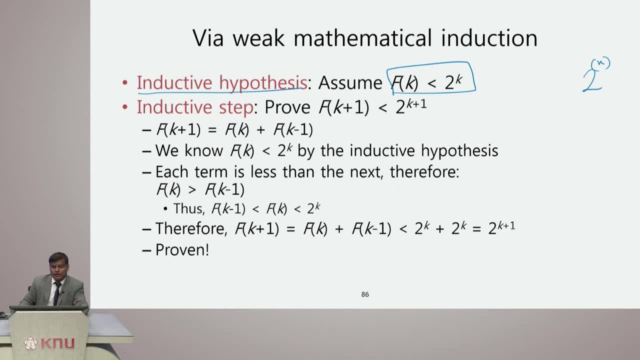 we have to prove for 2 power k. We assume that we have, we assume that it is true- for 2 power k. And then we have to prove for 2 power k plus 1.. That is where we finally. 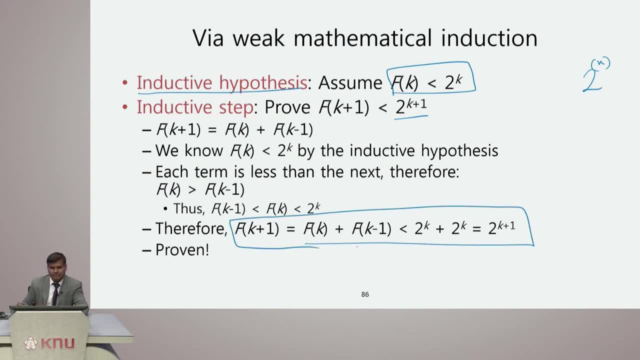 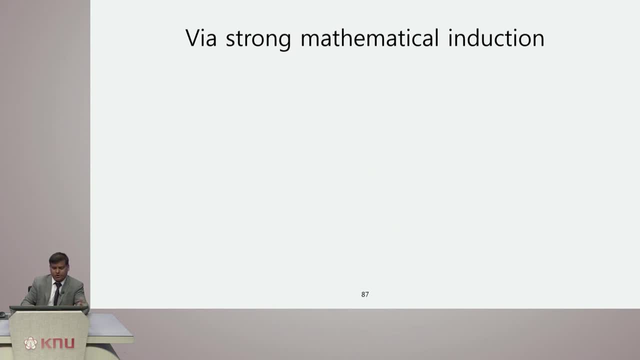 proved for 2 power k plus 1.. So this is the overall proof that we have via mathematical induction. And how about strong induction? Strong induction, as you know that we have to show for all values: f of 1, f of 2,, f of 3,. 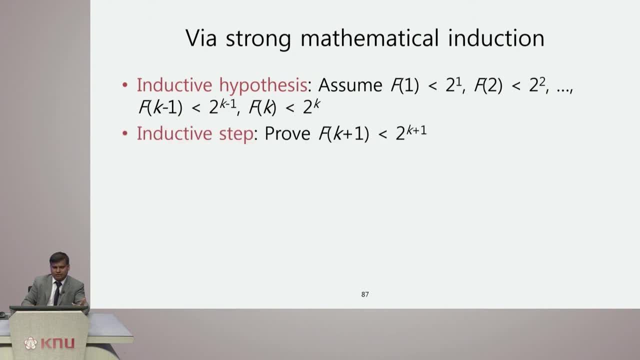 till f of k And then for inductive step we take that f of k plus 1. What is the next value? So initially for inductive hypothesis, we do not have to prove all values, But for inductive step. 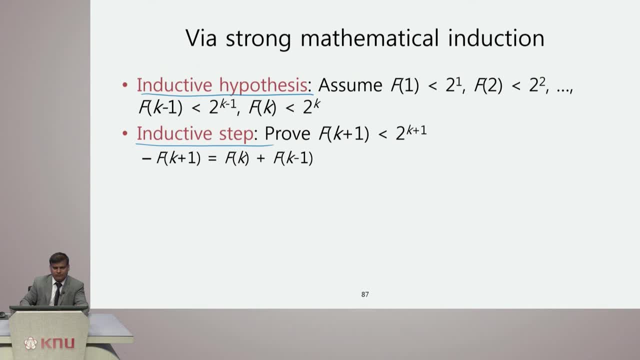 we have to show So here. f of k plus 1, equals f of k plus f of k minus 1.. So we know that f of k is less than 2 power k by inductive hypothesis. But that is one of the assumptions. 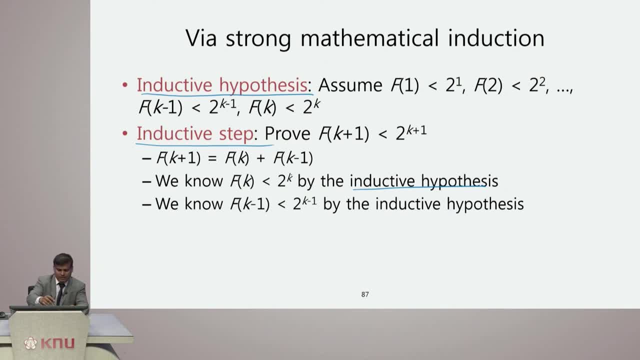 that we have there. So with this in mind, we can apply this that values over here. So f of k minus 1,- therefore f of k plus f of k minus 1, is less than 2 power k. 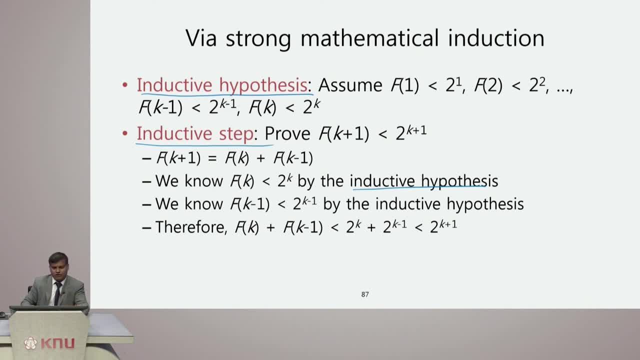 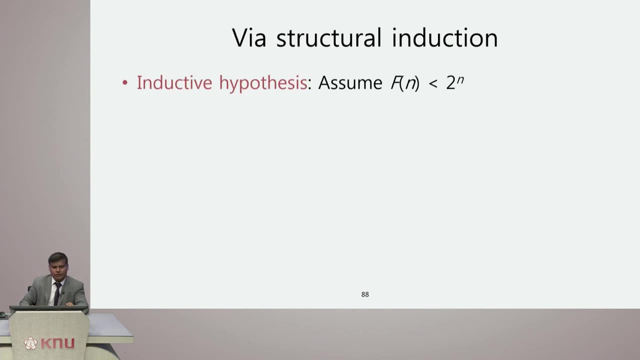 plus 2 power k minus 1, is less than 2 power k plus 1.. So that is that is it. We have proved here for inductive step Why a structural induction, That is, recursive steps. So we have this inductive hypothesis. 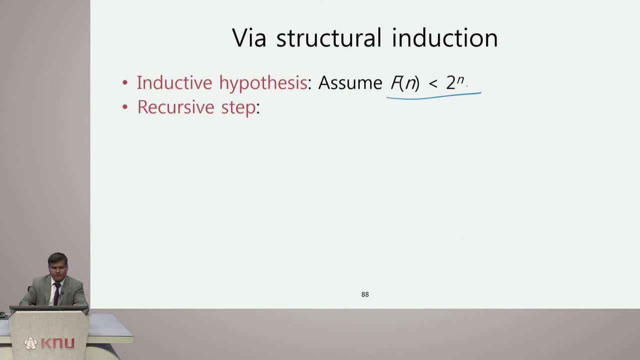 We assume that f of n is less than 2 power n. This recursive step in which we have to show it is true for a new element, n plus 1. We assume that it is true for the old element. 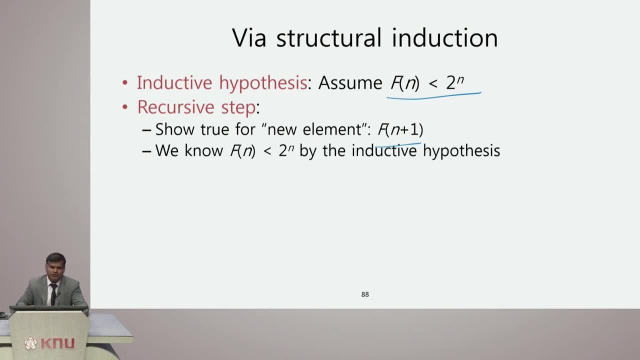 n and we have to prove for the new element n plus 1.. So we know that f of n is less than 2 power n by inductive hypothesis. That is the assumption. We know that it is true. 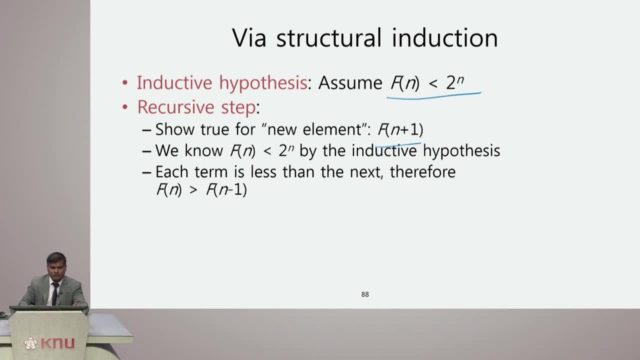 We know that f of n is greater than f of n minus 1.. Right The same principle that we have used earlier. We know that each term is less than the next term, So by that we are saying f of n is greater than. 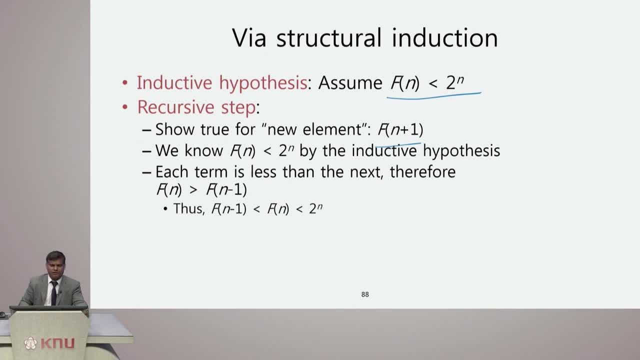 f of n minus 1.. Thus, f of n minus 1 is less than f of n less than 2 power n. Using the same idea here, Therefore, we say that f of n plus f of n minus 1 is less than. 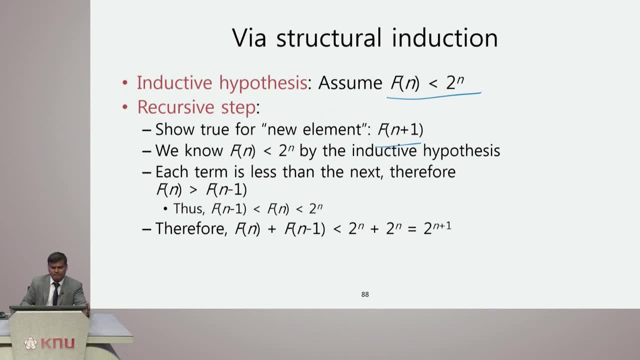 2 power n plus 2 power n, That is equals 2 power n plus 1.. So if you want to, of course, last two induction methods as well as the first one, you can have a look at your ideas. 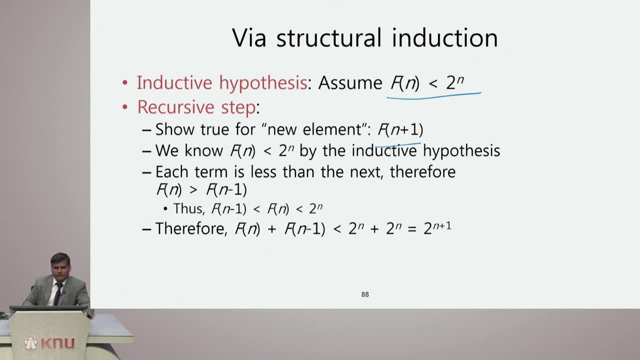 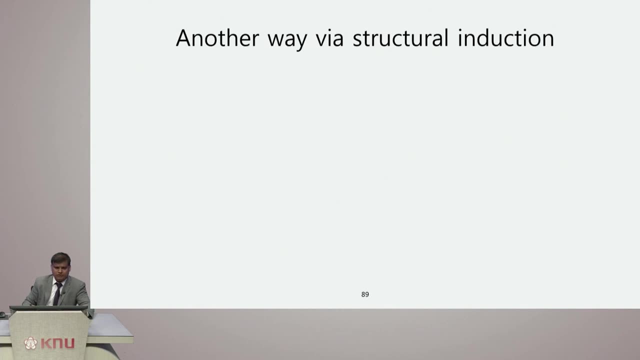 Just for your thought, you can just have a look at what is going on from the beginning And you can see how this whole proof has been defined. So thus we have been proved it. So another way we are going to use. 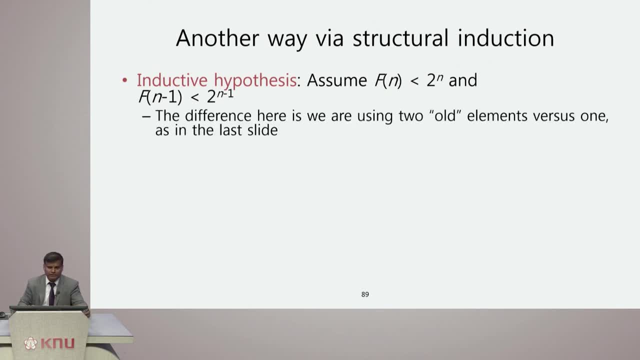 f of n minus 1 is less than 2 power n minus 1.. So that is the previous term there. The difference here is that we are using the two old elements versus one, as in the last slide. So in the last slide. 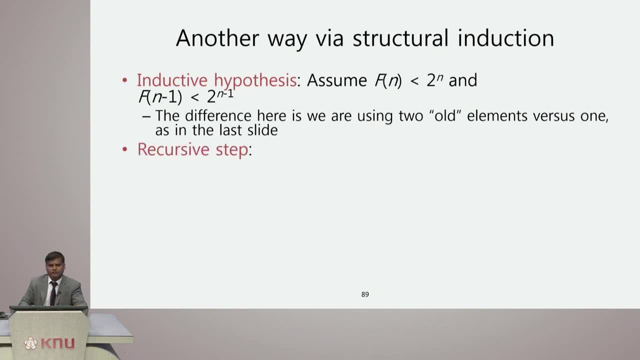 we just used one previous element, but here we have f of n is the old element, which is true for the new element, f of n plus 1.. We have n minus 1, we have n and n plus 1.. n and n minus 1 are: 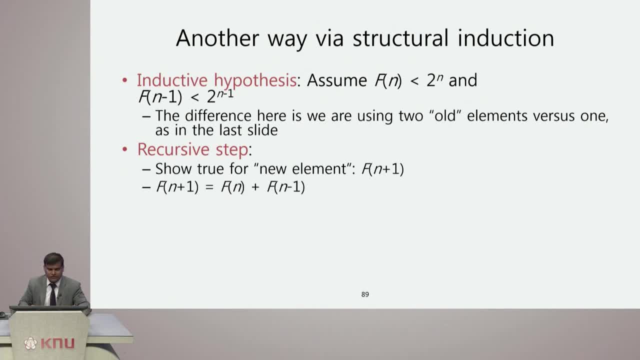 the old elements. So we are going to use those to prove it. So f of n plus 1 equals f of n plus f of n minus 1.. So we know that by Hindertree hypothesis we know that f of n is: 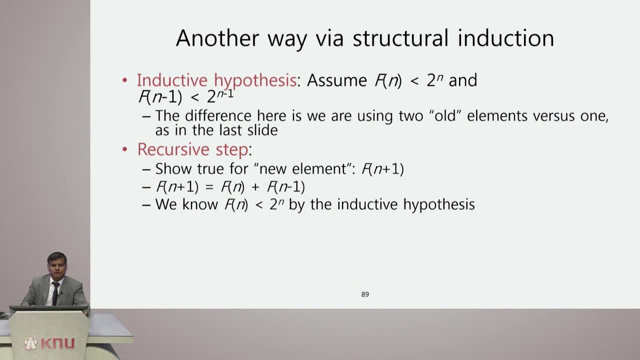 less than 2 power n. That is true. So we know f of n minus 1 is less than 2 power n minus 1 by Hindertree hypothesis. Again, that is another old element, So we know that that is true. 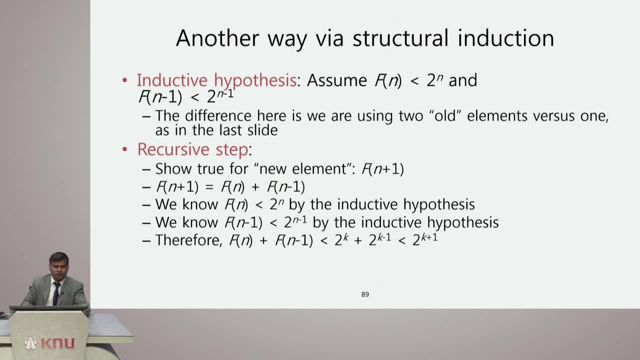 Therefore, f of n plus f of n minus 1 is less than 2 power k plus 2, power k minus 1. That is less than 2 power k plus 1.. Thus it is proved. Well then, now let us. 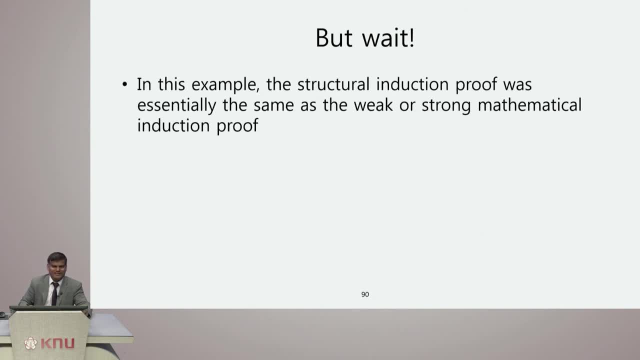 go for a thought here. So this example, the structural induction proof, was essentially the same as weak or strong mathematical induction proof. So it is hard to find an example that works well for all induction types. It is not that much easier. 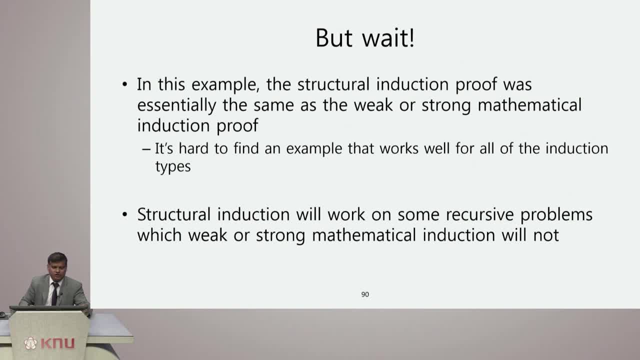 But structural induction will work only not only like structural induction will work on some recursive problems. So that is one of the advantages where which the weak or strong mathematical induction will not work on it. So as far as we have seen, 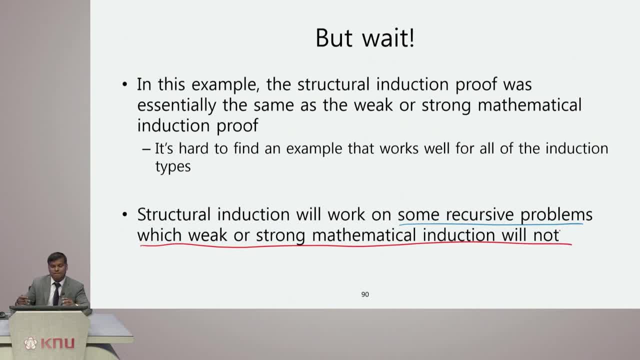 the structural induction will work on some recursive problems, whereas the weak or strong mathematical induction will not work on it. So that is the thought of the day. So today we have seen about the recursion. So as far as the structural induction is concerned, 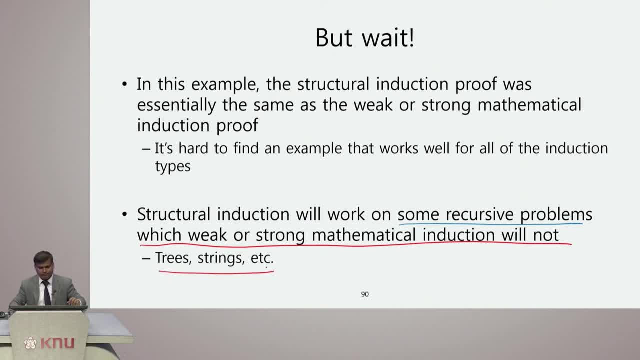 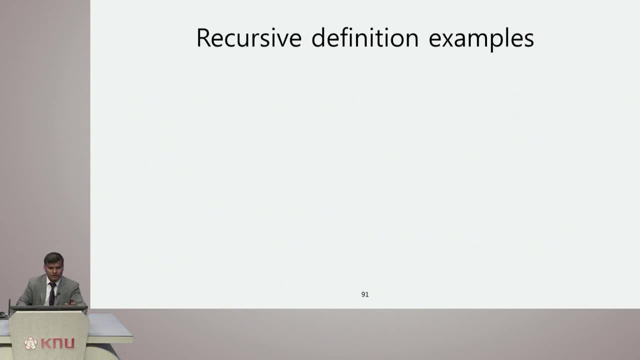 things like trees, strings. we can go for structural inductions And, as we have seen today, lot of interesting topics about recursion in general. So let us basically have this recursion definition. examples like: give this recursive definition of following sequence: Note that many 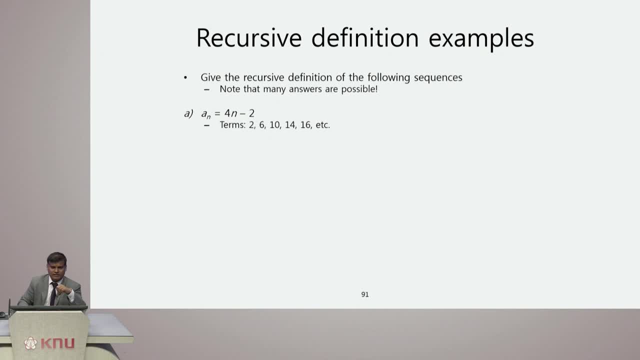 answers are possible for the following sequence: a sub n is equals 4 n minus 2.. The terms 2,, 6,, 10,, 14,, 16, etc. can be obtained For a of a sub 1 equals 2.. 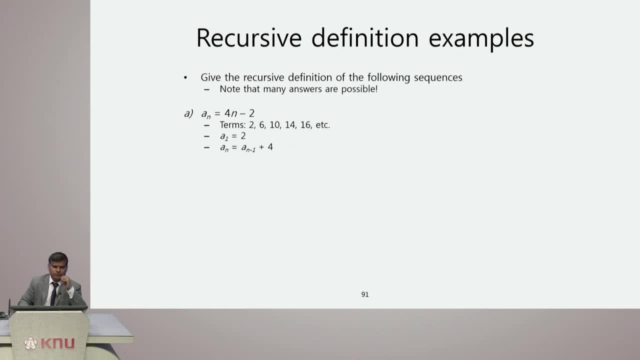 a sub 2 equals 6 and so on. So a sub n equals a n minus 1 plus 4.. We have b, another recursion, you can come up with: a sub n equals 1 plus minus 1. power n. 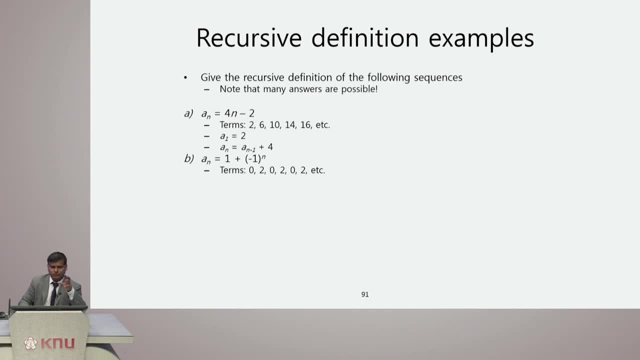 So we have the term 0, 2,, 0,, 2,, 0, 2,, etc. as being formed, In which a1 equals 0, a2 equals 2.. So again you have this: a sub n equals a. 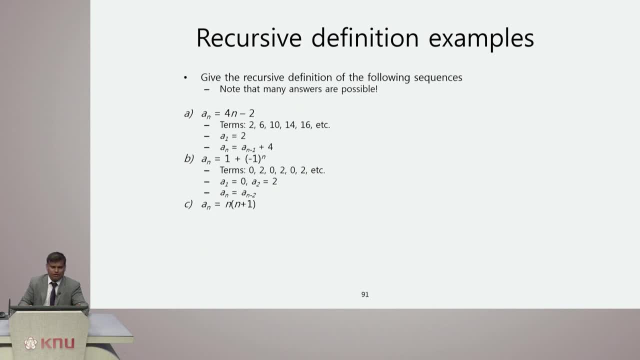 sub n minus 2, the form. So third one is a sub n equals n times n plus 1.. So we have the term 2, 6,, 12,, 20,, 30,, 42,, etc. So we have a1. 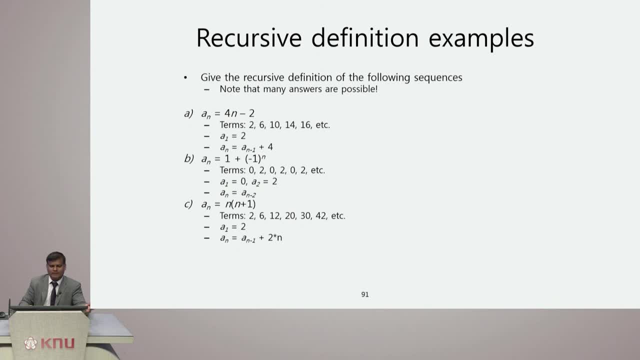 as 2, then an equals an. I mean a sub n equals a sub n minus 1 plus 2 times n. Then we have another one: a sub n equals n square. So we have 1,, 4,, 9,, 16 and 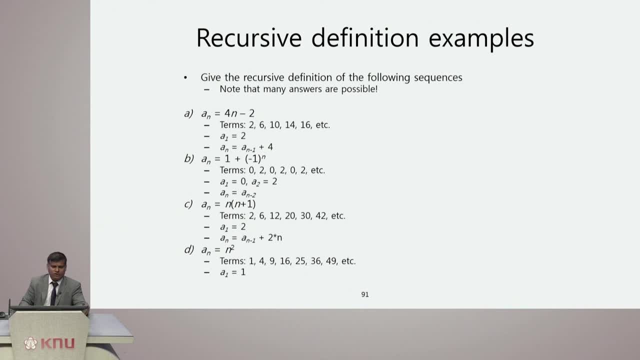 so on for the squares. So a1 is 1 and an equals a sub n equals a sub n minus 1 plus 2, n minus 1.. So these are some of the basic definitions, basic, simple examples for what recursion is given to us. 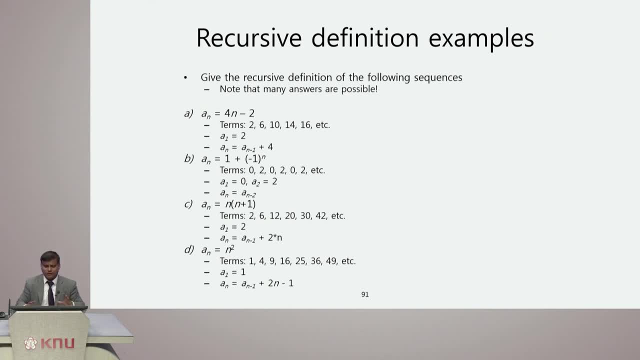 So, generally speaking, the things that we learned today all has to do with the recursion. We know what is the advantage of using recursion and you know what is the disadvantage of using recursion, And we know we should be very cautious of using recursion because at times we might go. 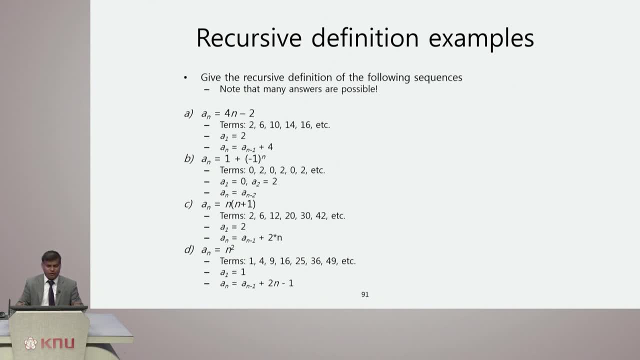 into some deadlock state. And now you have found the relationship between the recursion and the weak as well as strong induction. So as we go with this recursion step, we call this kind of proof as structural induction. So structural inductions are good for.